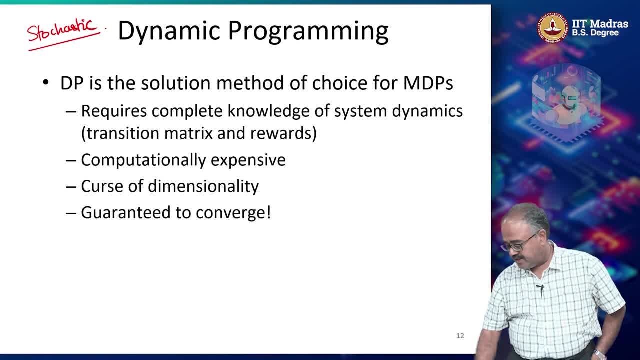 state and action value functions associated with the policy pi. So we looked at already. so V pi and q pi, these are policies associated with a specific- sorry, these are value functions associated with a specific policy pi. And then we also saw v star and q star, which are: 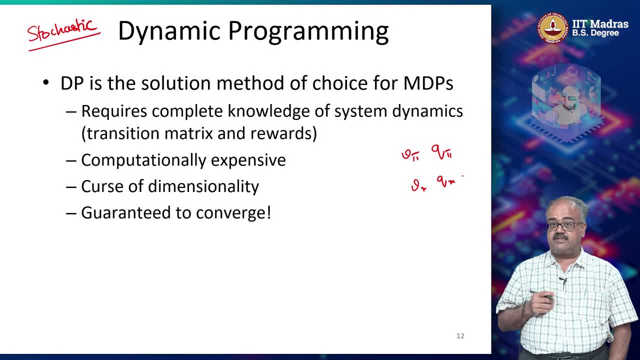 value functions associated with optimal behavior, or the optimal value functions, And so what we will look at is the first cut solution approach is to look at dynamic programming based algorithms for finding both v pi and v star or q star. So that is where we will. 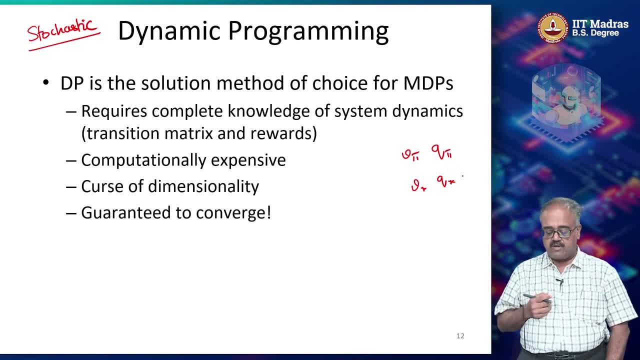 start off and then slowly we will relax our requirements as we go to solving the MDP. So just a side note here. so the problem of going from a pi to v, pi is called the evaluation is called evaluation. I am taking policy pi and I am evaluating it and finding out what. 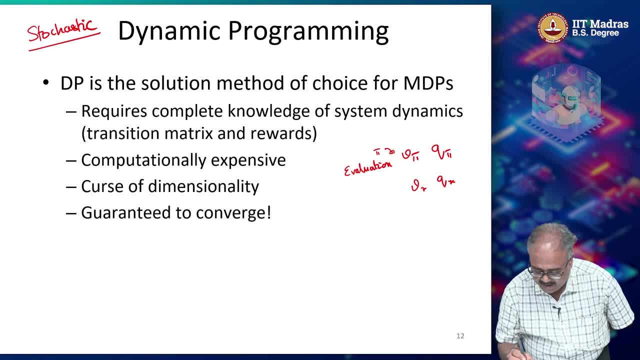 is the value function corresponding to the policy pi, And finding v star is sometimes called the evaluation Control problem. so the finding v pi is called the evaluation or the estimation problem. So finding v star or q star is called the control problem. So we can use dynamic programming. 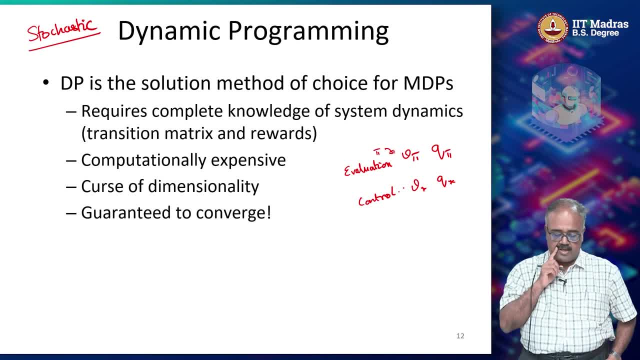 approaches for solving both evaluation and control. So the classically- classically when people have been talking about Markov- addition processes. so MDPs appear a lot in domains such as operations research and in sequential decision making and those kinds of areas MDPs appear a lot, They are used quite extensively there In fact. 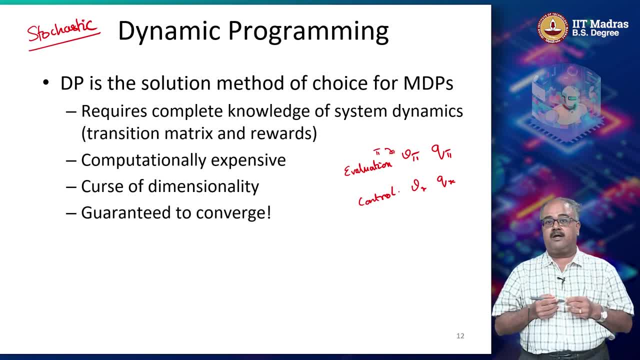 reinforcement learning borrows all the notions from operations, research and allied fields, So there, dynamic programming is the solution method of choice for MDPs, So this is what people use extensively. More recently what has happened is that reinforcement learning in turn has started influencing how people use dynamic programming for solving MDPs. 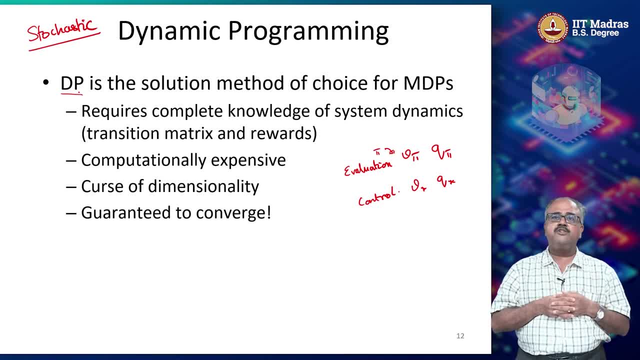 So we will. I will make allusions to it as we look at these topics in the later classes. We are not going to get into quite too much detail on that, So there are a few things that we should know about dynamic programming methods, As you. 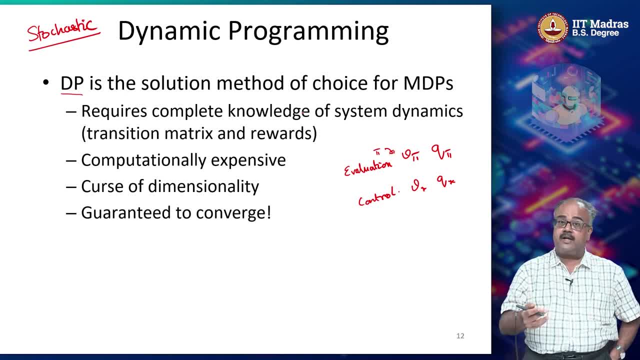 will see in a bit. they require the complete knowledge of the MDP. You need to know the states, you need to know the actions, you need to know the transition matrix and you need to know the rewards. So the transition matrix is what You need: to know the boundaries and so you know the. 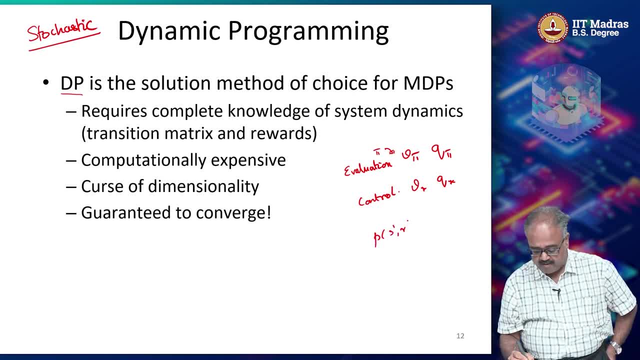 requirements. You need to know the limitations of an MDP and you need to know the rewards, need to know, basically, you need to know P of S prime, R prime given S comma A. that you need to know. or you need to know P of S prime given S comma A and the expectation of R given. 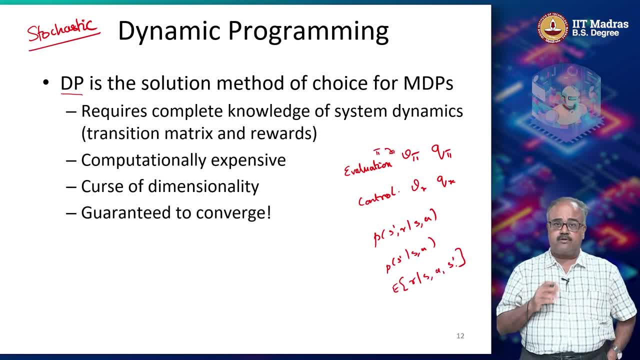 S A S prime. So these are, these are things that you need to know. this is what we mean by saying complete knowledge of the system dynamics and dynamic programming can get computationally very expensive. In particular, every iteration of the dynamic programming can be very computationally. 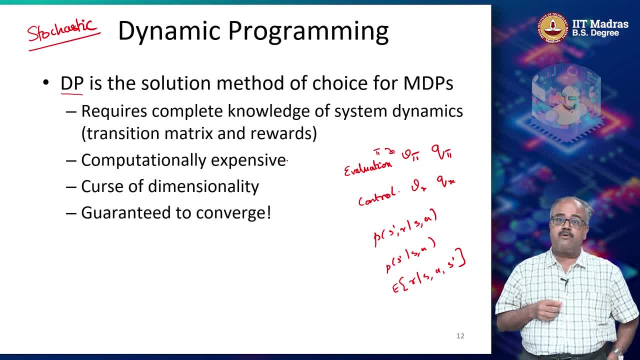 expensive, So the compute load, the peak compute load, can be fairly high. But the positive side, most of these dynamic programming approaches, under the right conditions they are guaranteed to converge. So this is a big plus. So you know that if you run these long enough, they 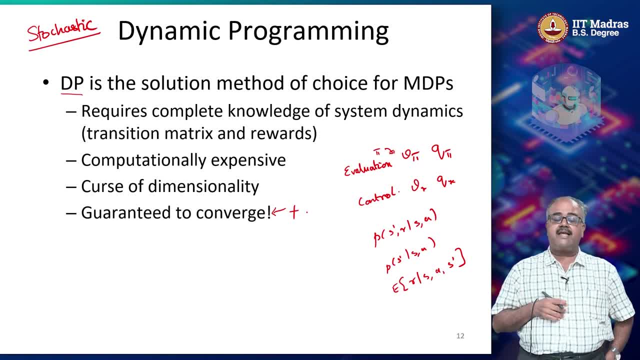 will eventually converge Under the right conditions. So this guarantee is unfortunately not available for all kinds of reinforcement learning approaches. even though they work well in practice, we still do not know if they will always work or if there are conditions under which these algorithms might not work. This will come down the line, So let us not worry about it too much. But 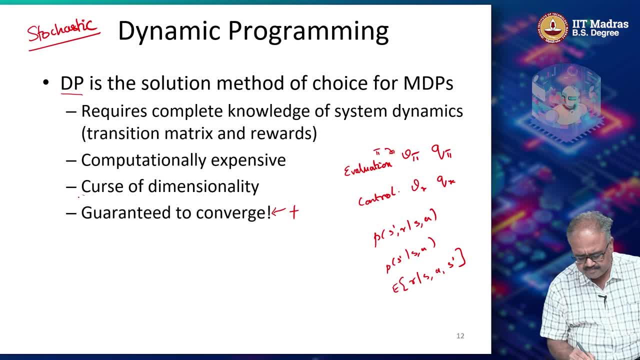 then there is also this thing which people call as the curse of dimensionality, And the curse of dimensionality is present in all the algorithms. So the curse of dimensionality is something that you call as the curse of the state space. So let us not worry about it too much, But let us not worry about it too much. So let 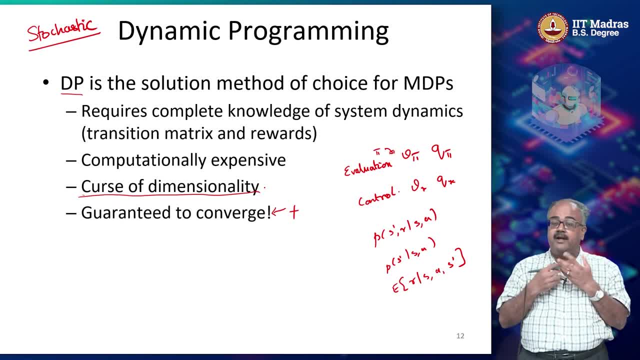 us not worry about it too much. I mean, the curse of dimensionality is very common for all approaches. It is more a question of how large the state space becomes. So earlier we looked at the simple MDPs, We looked at this kind of grid world. So where you had 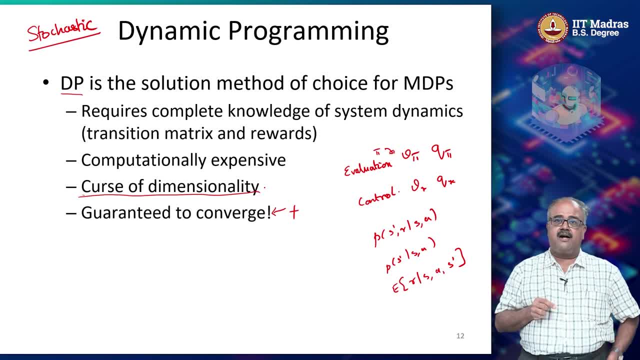 an x coordinate and a y coordinate and you are numbering the states in order. So if it is a 5 by 5 grid world, you will have states running from 1 to 25.. You could also think of that as two dimensions, So one dimension having 5 values, another dimension having 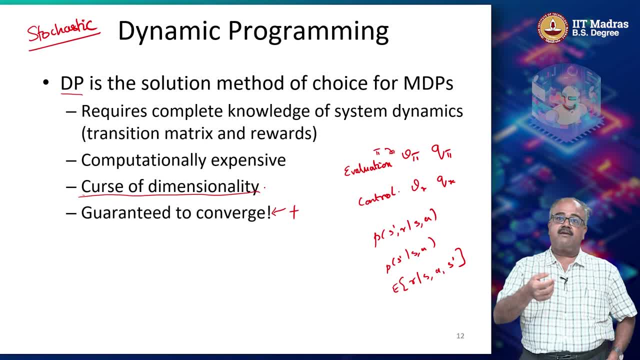 5 values, have 25, but suppose you have like 30 variables that are describing your system, right? not just the x, y dimension. I remember the robot example I was telling you about. right, there are multiple sonar readings, bump, bump sensors and and motor values and so on, so forth. right, torque values. 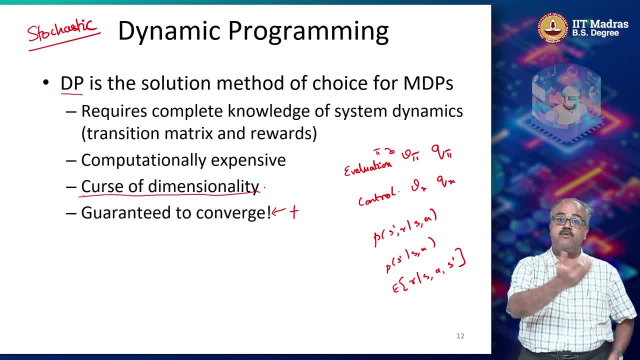 joint angles and all of these. so there are so many, so many different factors that can contribute to defining the state space right now. if you think about a transition matrix right in that large state space definition, so you will soon find that the system specification becomes very, very large. 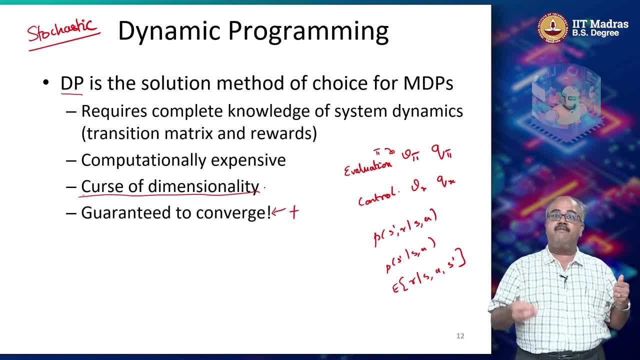 right. and if you add just one more variable, even if it is like a boolean variable, right, you kind of, you know, make the state space grow very large, right? so that is the that is a problem, right? so this is what we call as curse of dimensionality. so the larger the number of dimensions, that 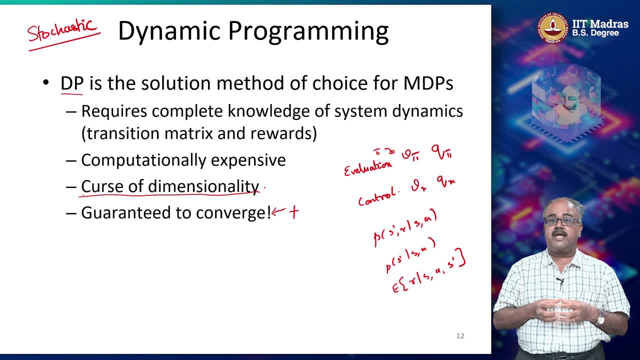 describe the space the the more you know exponentially there is the size of the state. space grows and therefore it makes it prohibitively expensive even to write down the system dynamics in in in analytic form so that you can use it for dynamic programming approaches. so that makes that makes dynamic programming fairly hard to scale for very large. 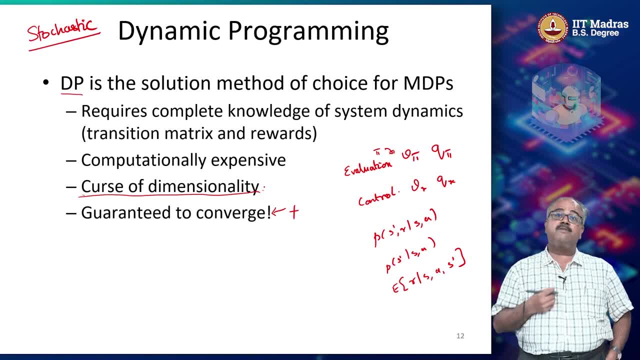 problems and methods that work without a complete specification of the system. dynamics scale much better, and we say that they do not suffer from that much, from curse of dimensionality. so that is essentially what what we mean by curse of dimensionality here, and so that is actually sometimes mentioned as one of the drawbacks of using dynamic programming. 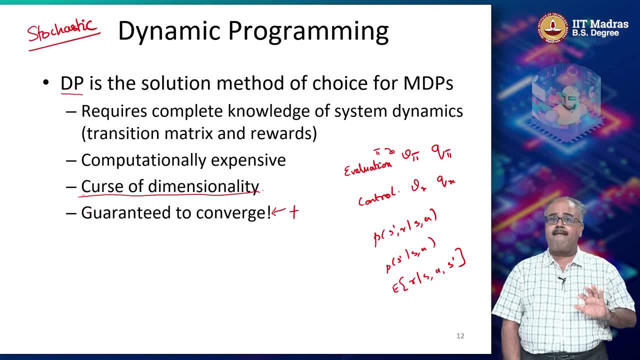 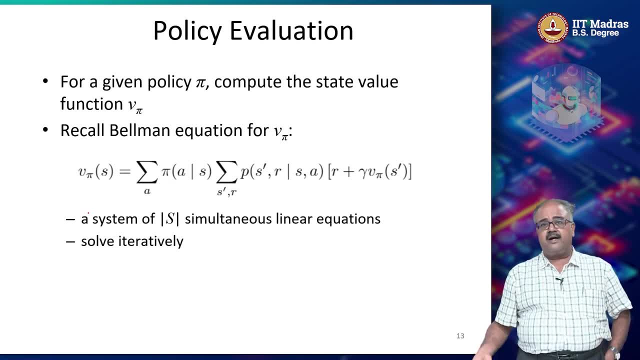 like approaches to solve entities, so there are ways of getting around it, but fundamentally, there is a problem that we have to think about. okay, so let us look at the first example. right, so we are going to talk about policy evaluation here. we are going to talk about the policy. 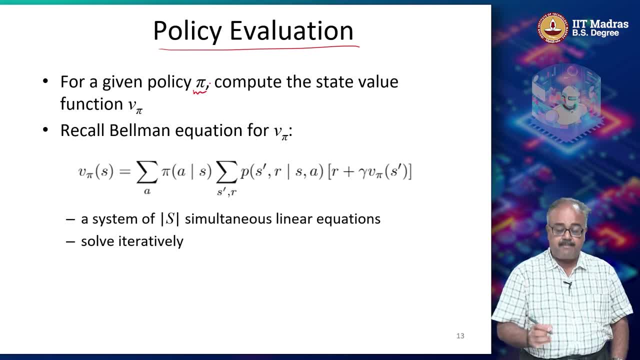 evaluation step. so policy evaluation is given a policy pi. right, you want to compute the state value function v pi. given a policy pi, you want to compute the value function v pi. okay, so how do we go about doing this? recall that we have the bellman equation for v pi. 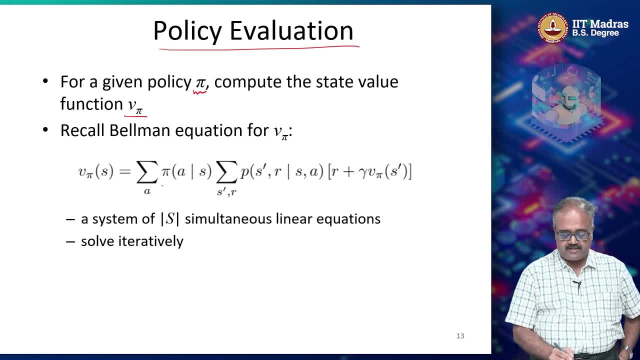 right. so what is the bellman equation for v pi? so v pi of s is equal to, you know, the summation over a, summation over s prime and r, the summation over a of pi a s, a given s and summation over s prime and r of p of s prime. 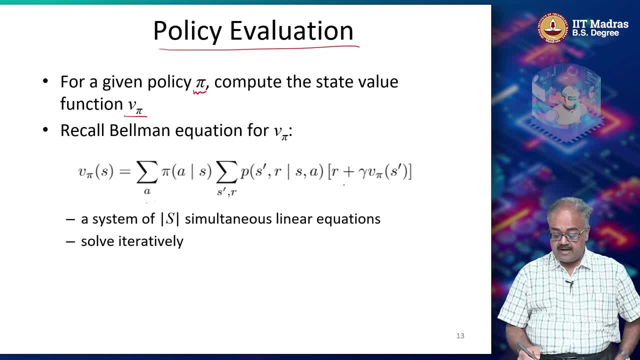 given r- i am sorry- s prime and r, given s comma, a times r plus gamma v pi s prime. okay, so this is the bellman equation for v pi. so we know that we have seen this already. we know how to derive this and all that. so how are you going to solve for this bellman equation? so what is the bellman equation? 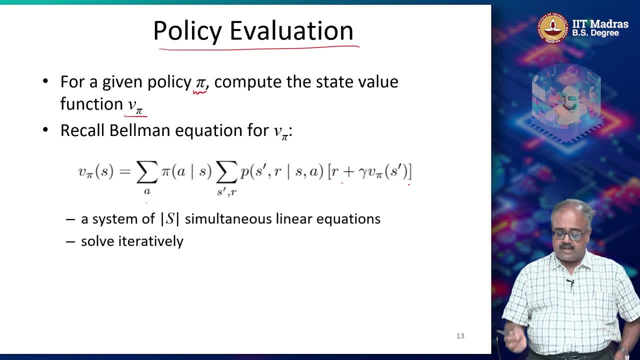 So what we mean by solving for this Bellman equation. so what are the unknowns here in this Bellman equation? Again, this is more of a recap. The unknowns here are: the v pi is right. So the v? pi is unknown. So you have v pi of s on the left hand side of equation. 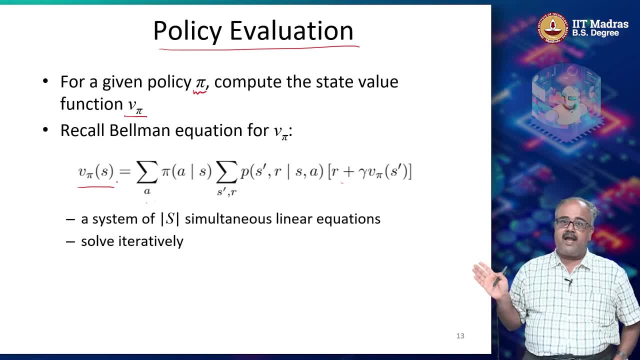 you have v pi of s on the left hand side of equation and you have v pi of s on the right hand side of the equation also. So what do we mean by that? So you have V phi appearing here. So this is an unknown. this is also the unknown, and the same S can appear here also. it is not. 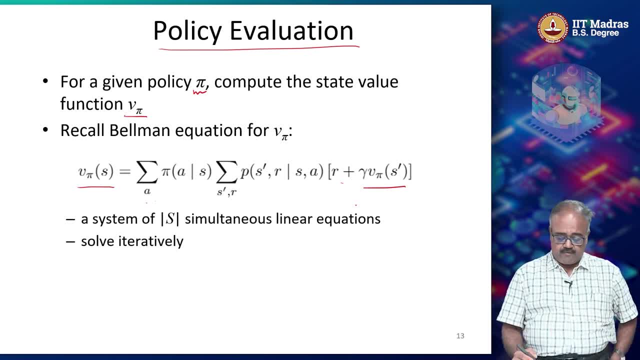 like it will appear only on the left hand side. So now, if you think of it, I am going to have, let us say, the size of my. so my state is S, the size of my state. space is denoted by that symbol. 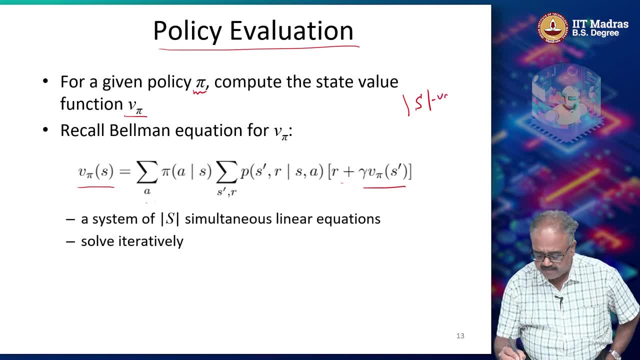 So that is the size of S and I will have that many variables. So I have one V phi of S for each S in capital S. So I have size of S, number of variables. let us, for convenience, let us say: 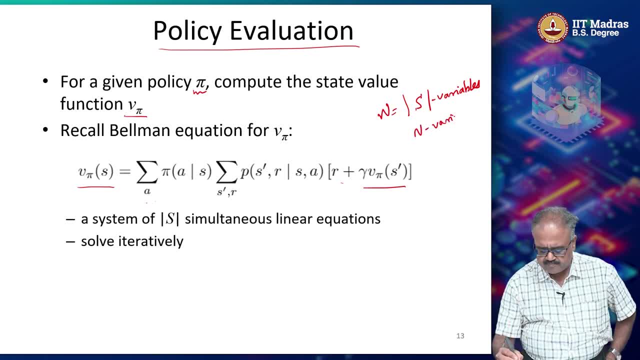 this is n, So I have n variables. and how many such equations I have? I will have one equation for each V phi of S on the LHS, So I will have n equations. So I have n variables. I have n equations. and what kind of equations are these? These are all. 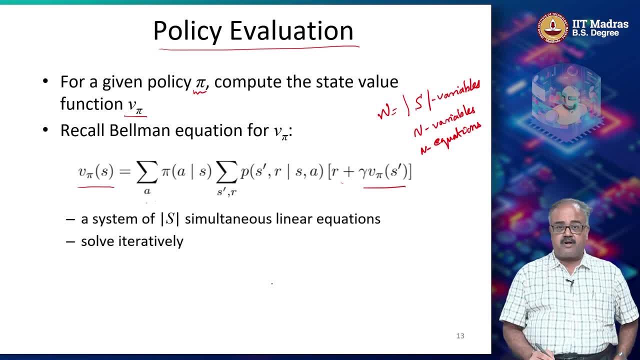 linear equations. Even though there are so many products that are happening here, at no point will you see a product of two of the unknowns. I am not going to see V phi of S1 times V phi of S2 or V phi of S1 squared anywhere. So these are all going to be linear equations. So 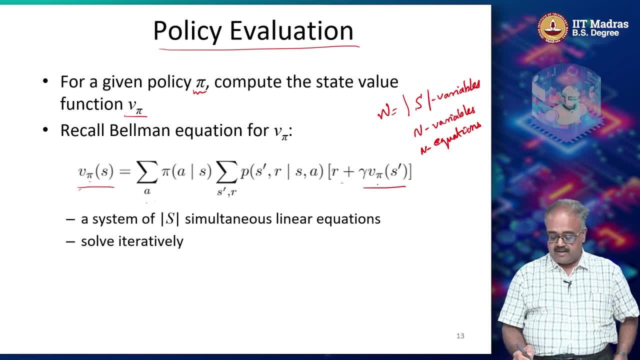 that is basically what we have here. So V phi of S, again V phi of S1, V phi of S. on the right hand side there are no higher order terms, So it is a set of linear equations. So there are n equations in n variables, So these are simultaneous linear. 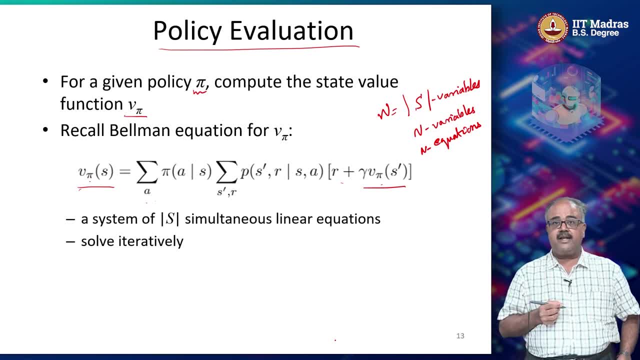 equations and you have lots of methods by which you can solve it, Provided you have the right degrees of freedom and therefore the solution is well defined. It turns out because of the way we constructed this Bellman equation as a way of representing how the value rollout happens, how the return is rolled out, as you are. 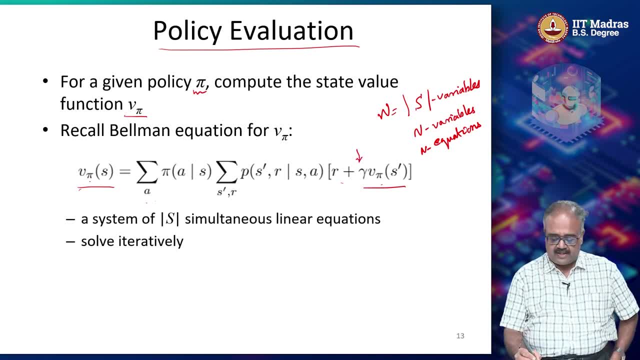 executing a policy, pi- and the fact that your gamma is a limiting factor. So gamma is between 0 and 1.. So this put together actually ensures that not only does the system of linear equation have a solution, it also ensures that they have a unique solution. there is a single solution for it. 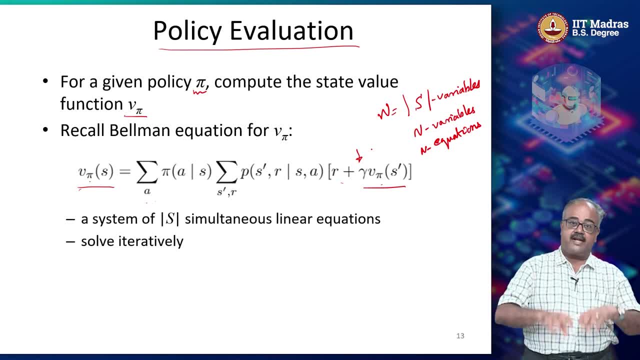 So for each policy pi there is only one solution that satisfies the Bellman equations. We talked about this earlier And there are some videos that you can refer to that will be linked as part of the additional reading material, So these videos are not. 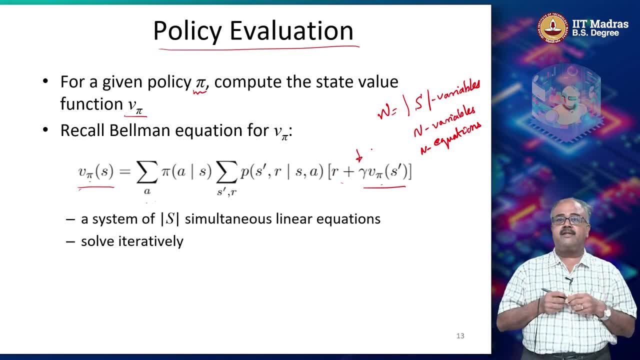 required material. So if you want to understand why there is a unique solution to this V phi, you can watch those videos So you could solve these like simultaneous linear equations. system of simultaneous linear equations. There is another interesting way of looking at this. So this is where the 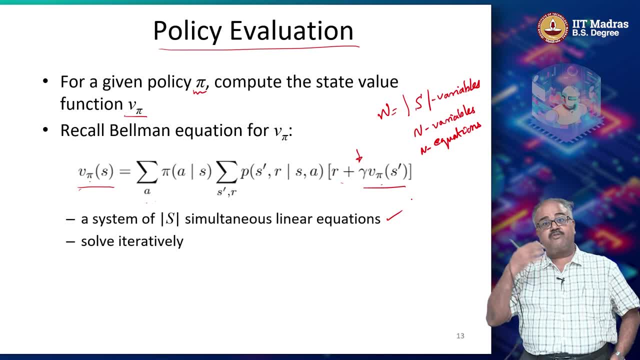 dynamic programming part comes in, And also this is an approach that we will use lately when we are trying to compute the optimal policy also, not just the. the optimal value function not just for e pi. You could solve this whole thing iteratively. 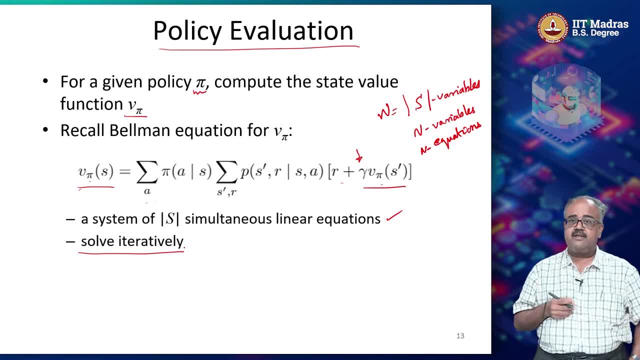 So how do we do that? So let us take a look, how do we do that. So I am going to start start doing this iteratively. So what I will do is I will take v0, that is so I am given. 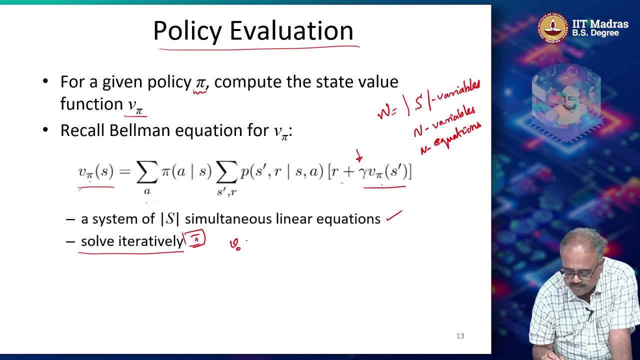 some policy pi. that pi is fixed. So I will take v0, I will define it uniformly to v0 for all s. I will define this uniformly to be 0 for all s. Now I will plug in vk to the right-hand side and compute vk plus 1 on the left-hand side. 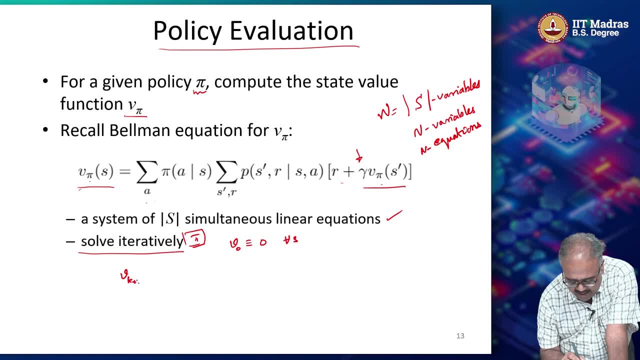 So it is going to go something like this. So it will be: vk plus 1 of s is equal to summation over a pi of a given s, summation over s prime comma, r p of pi of a given s. So this was a little complex to solve because I had unknowns on both the left-hand. 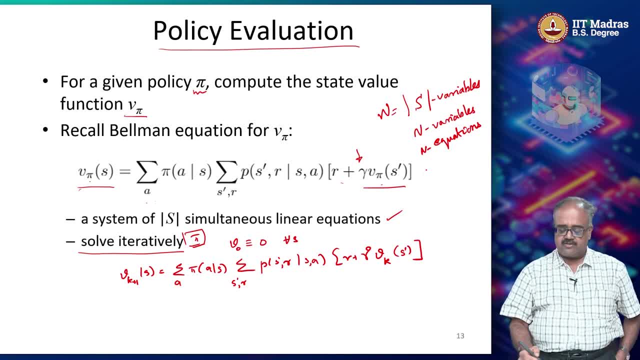 side and the right-hand side. Now what I have done. I have rewritten it so that on the right-hand side I have k, on the left-hand side I have k plus 1.. So k plus 1 are the. 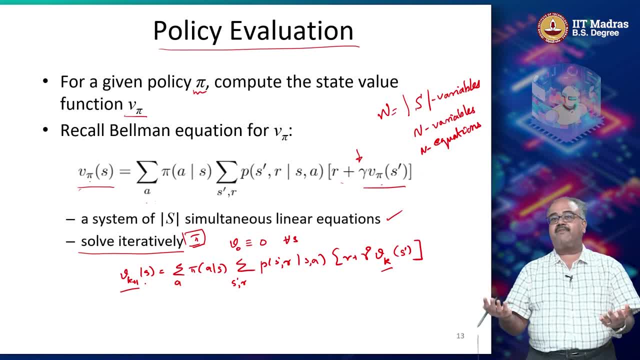 unknowns. So vk plus 1 are the unknowns. but on the right-hand side I have everything that is known because I already computed vk. So how do I do that? I start off by defining v naught equal to 0.. I start off by defining my v naught equal. 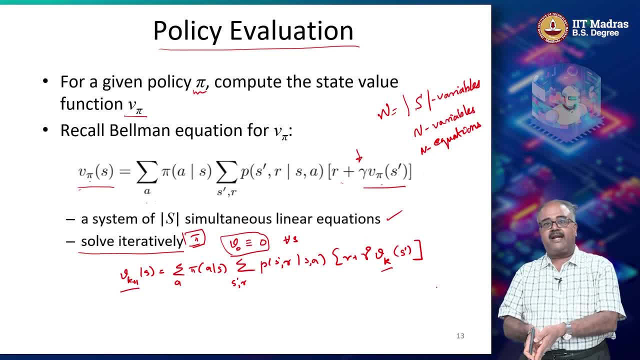 to 0.. And then from there I am going to plug in my v naught on the right-hand side. Now, everything is known on the right-hand side. If I plug in v naught on the right-hand side, everything is known on the right-hand side. Now, what I will do is I will compute v1.. 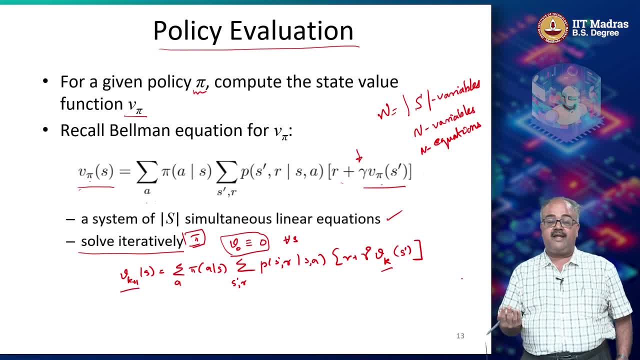 And then what I will do. I will take v1, I will plug it on the right-hand side and I will compute v2.. Then I will take v2, plug it on the right-hand side, compute v3. So I keep doing this until so when I go from some very large Vn to Vn, plus 1 or so Vk to. 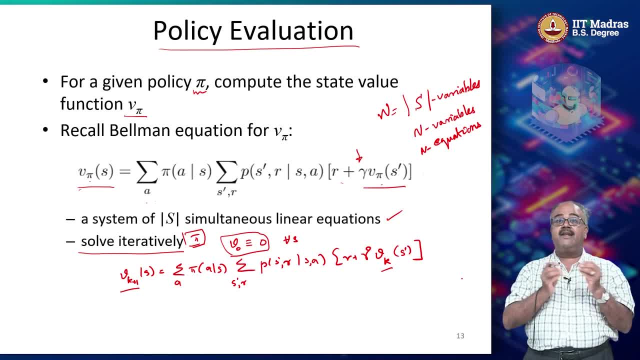 Vk plus 1. for some very, very large k there will be very little change. Vk will look very similar to Vk plus 1.. At that point I stop. There could be some very, very small, say 10 power minus 3 difference between Vk and. 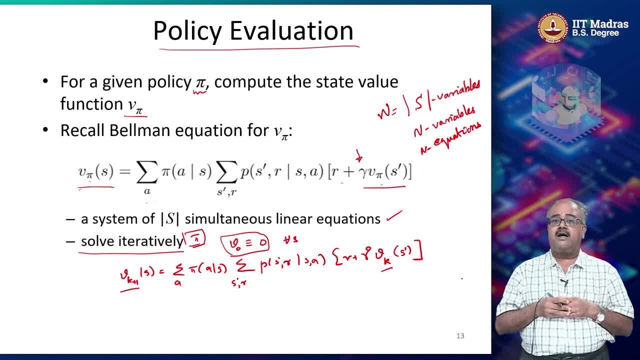 Vk plus 1.. At that point I can stop my iteration and declare that this is my V? pi. So it is really. you could think it is a little wasteful. Why am I doing this iterative process? I have a neat system of linear equations. 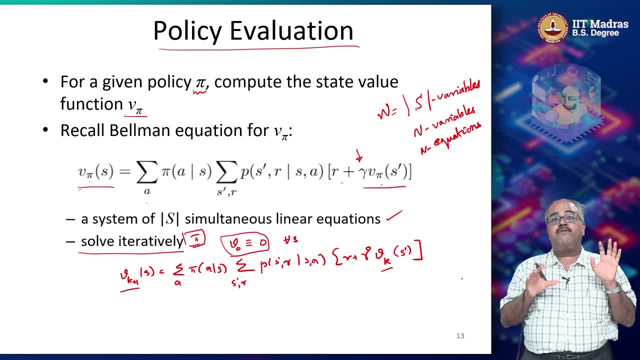 I can just solve it. It turns out this iterative process gives us a lot more flexibility in how we will arrange the computation and allows us to come up with more efficient ways of approximately solving the problem, While policy evaluation will solve the problem accurately but will end up taking a lot of. 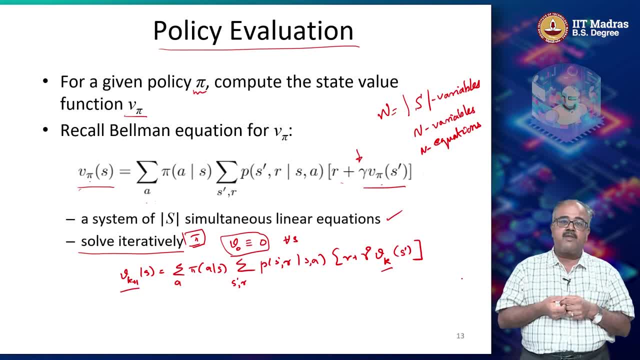 compute every time you go through this, while this kind of iterative approach might allow us to solve these things. So it is a little wasteful, But if I want to solve this problem more efficiently, I have to do it, And also I will act as a building block for finding the optimal value function as we 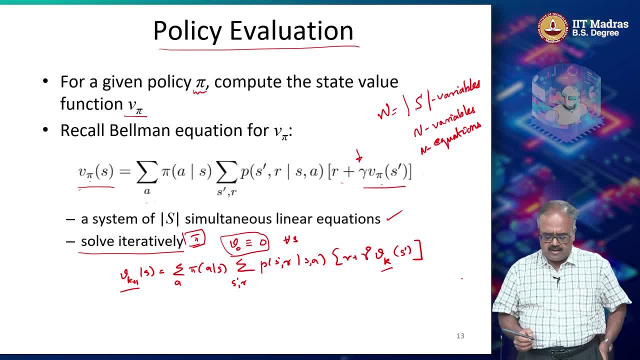 will see in a bit. So let us think about what is happening here. for one net, I start off with V, not equal to 0,, all 0s. So what will happen here? I will plug that in here. So for k equal to 1, so k equal to 0, start with k equal to 0, so what will happen is: 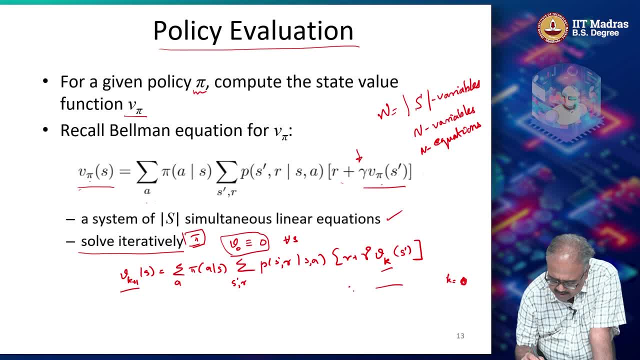 I will plug V not equal to 0. So this whole part will go away. So I will be just left with R. So I will sum over S prime comma R, probability of S prime R given S comma A, into R. summation over A pi of. 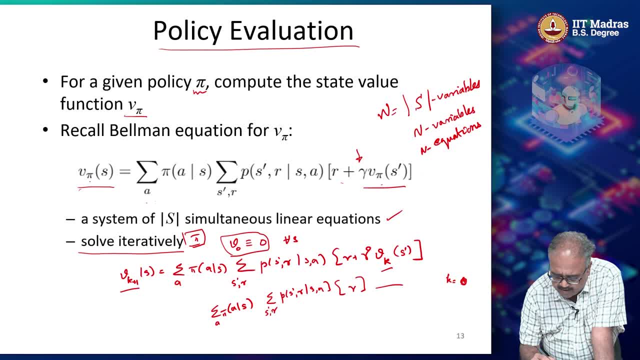 A given S. So I am summing over all S prime, so all possible values of S prime. So this is basically, and I am multiplying by the same R. So this is essentially saying that summation over R of probability of R given S, comma A, because, because I am summing over all S prime, 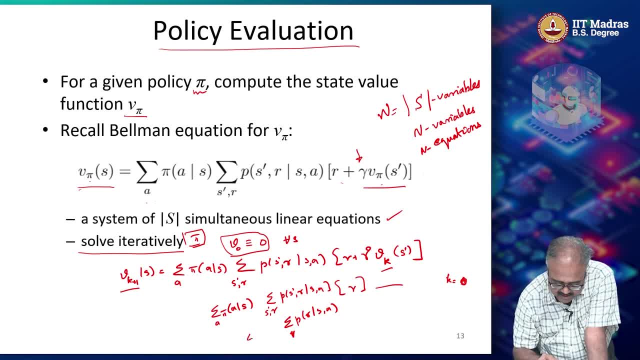 So that is going to go to 1. So, and then sum over A pi of A given S. So this is basically what I am computing. So what is this expression? This basically tells me I am going to behave. 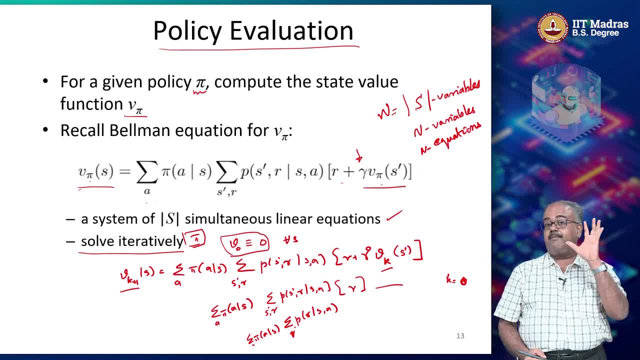 according to pi. pi, I am going to behave according to pi. I will take one action starting from state s. so that is what this is: I take one action starting from state s. look at what the reward I am going to get, the expected reward I am going to get, This is the expectation of the 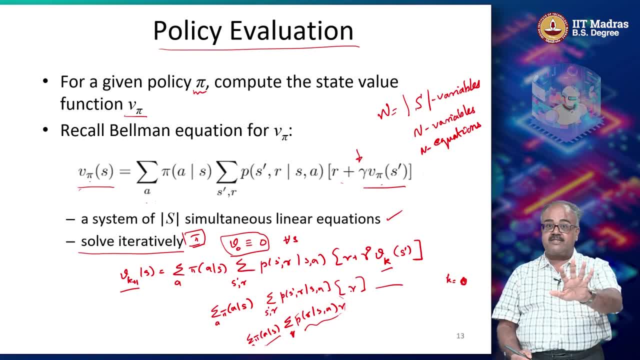 reward I will get for taking one step. I do not care where I land up because I am just done, I am just taking one step: get it. So this is basically v1 of s: I am just taking one step and I am looking at the expected reward when I am taking actions according. 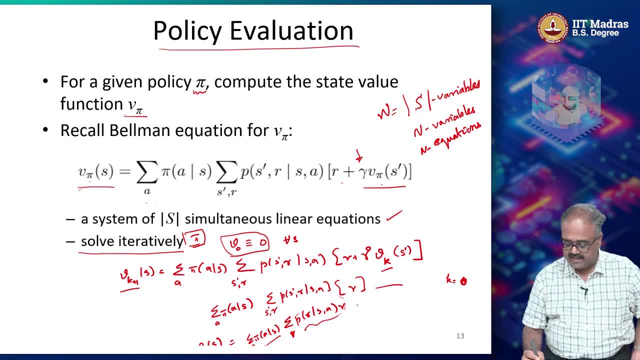 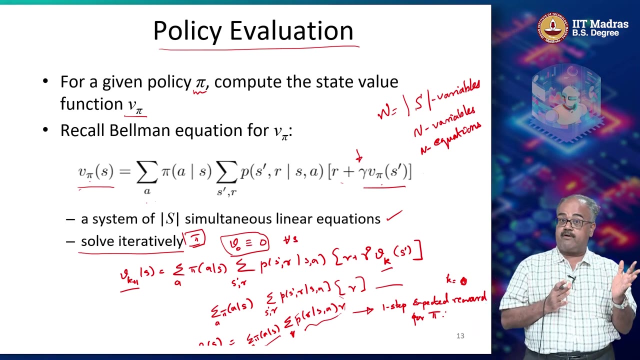 to my policy pi. This is basically what it says. is this is the one step expected reward for taking one step. Now what is v1 of s for policy pi? does that make sense? So v1 of s is essentially: 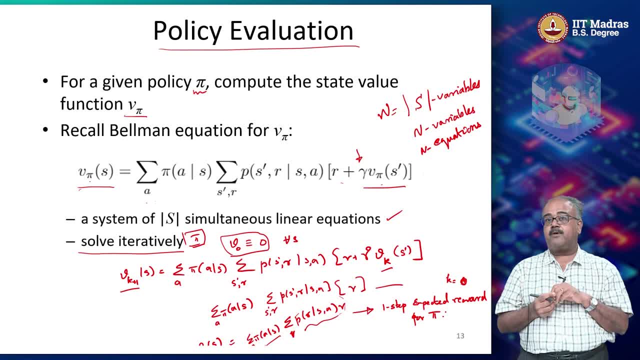 the expected reward I am going to get for taking one step according to policy pi And then extending this, you can think of v 0 of s as the reward that you will get for taking no steps. this is basically no reward, so that is why it started off with 0.. Now that 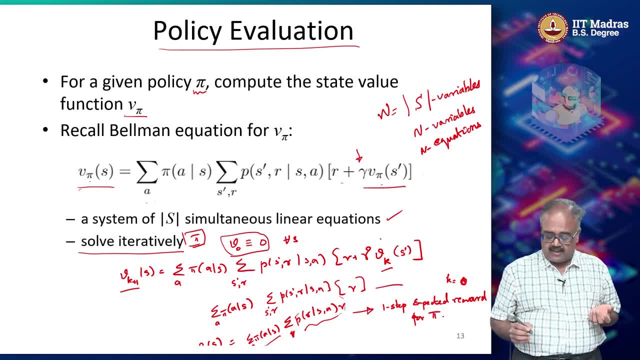 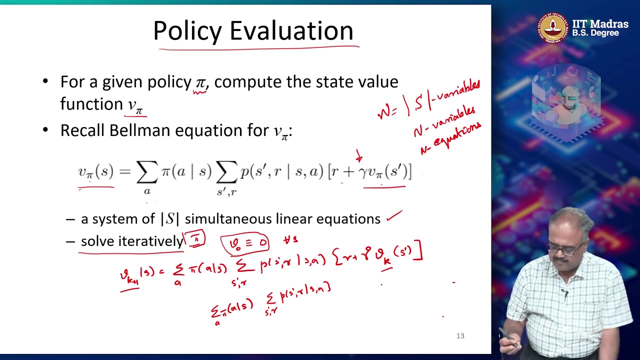 you have solved this for one step. I am going to plug that in to the right hand side. So let us. yes, for lack of space, I am going to erase this. I hope it is all fine with people. Now what? 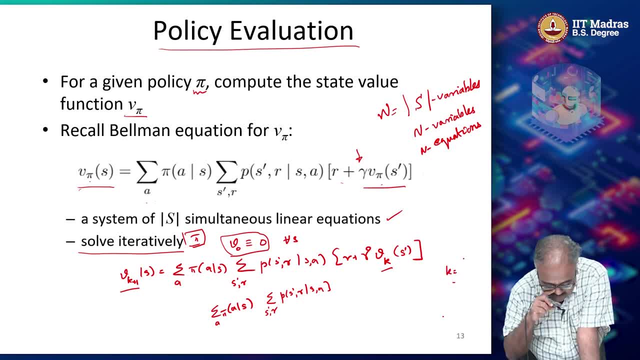 I am going to do is I am going to look at what happens when k equal to. so this I computed for k equal to 0.. What happens in k equal to 1?? So this will be r plus gamma v1 of S prime. That is basically just plugging in k into this expression. So what does this? 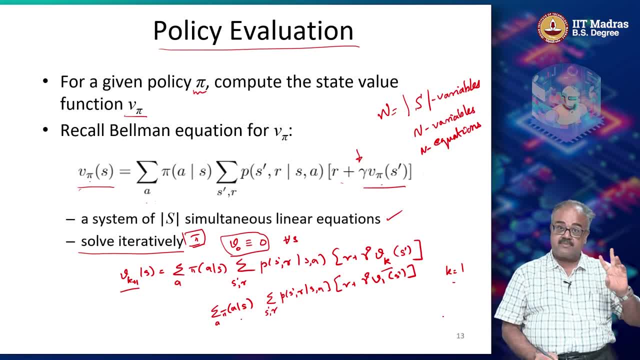 mean. So I am going to start from state S take action according to policy pi. Start from state S take action according to policy pi. I will go to some next state S prime. Then I look at the reward I get for going to the. 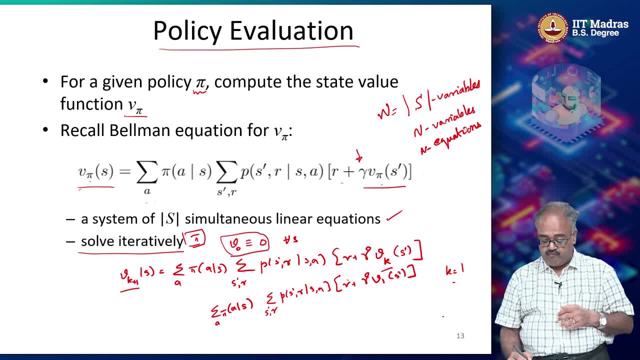 next state: S prime plus gamma times v1 of S prime. So what is v1 of S prime? This expected reward I am going to get for taking one step from S prime. v1 of S prime is the expected reward I am getting for taking one step from S prime, And r is the reward I am going to. 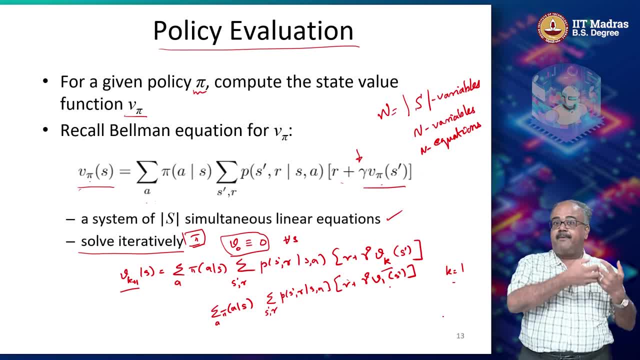 get for taking one step from S. Basically, what is happened is I am taking r plus gamma times, the reward for taking one more step from S prime. So, starting from S, how many steps have I taken? Two steps right. So when I say v2 of this, it is basically the two step expected returned from S with 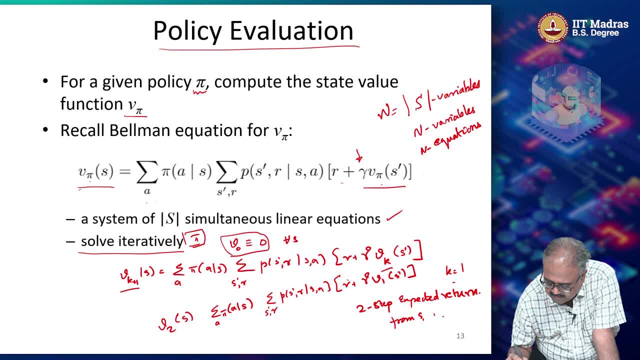 2 steps of r. Again, reduce that. okay, Yes, The policy being pi, because v1 of s s prime is already assuming you are taking actions according to policy pi from s prime. and here we are making the assumption you are taking action according to policy pi from state s also. 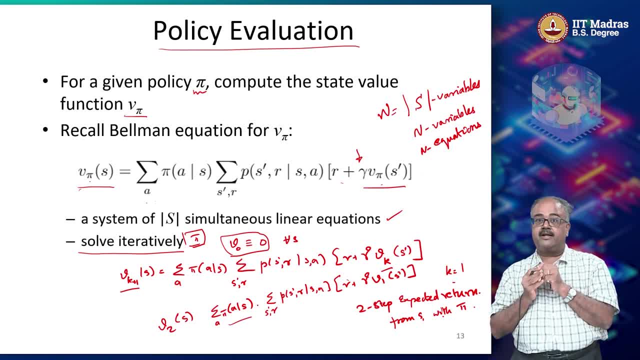 So now I have used my one step expected reward and use that to compute my two step expected return. So after I do not, I do not worry about what happens after my second step, it is just I am just shopping at the second step here. so that is basically the second iteration. 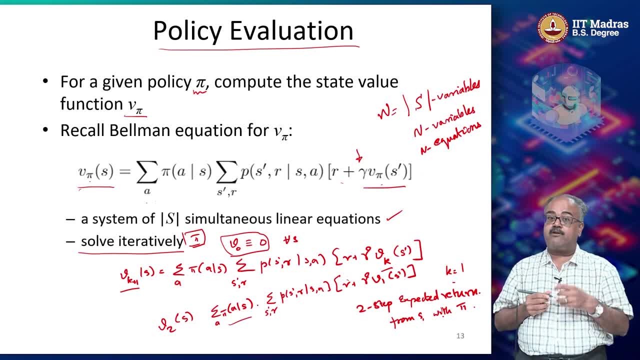 of my policy valuation. Likewise, what happens when k equal to 3, I am going to get my three step expected return. and if a k as k becomes larger and larger, I am going to get my, you know, infinite expected return. basically the complete expected return, starting from s unbehaving according to policy. 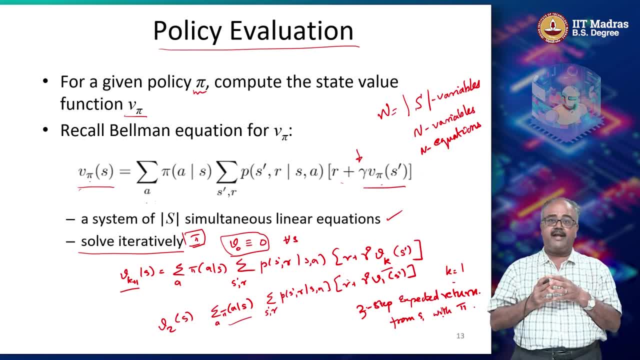 pi. So this is the basic idea behind the dynamic programming way of doing policy evaluation. that is why it is called dynamic programming, Because I first solved- I solved the zero step problem, which is the assumption making it all zero, and then I solve the one step problem, and then I solve- I use the solution I got for the one step problem. 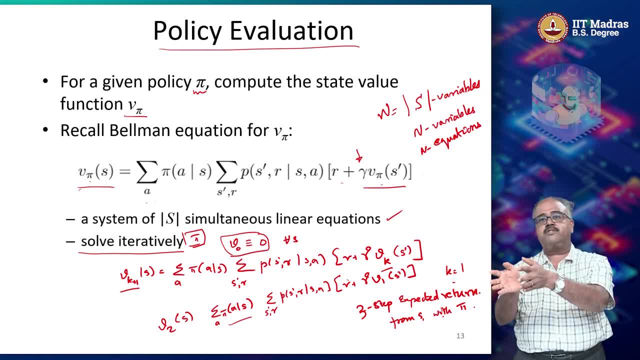 and solve the two step problem. then I got the solution I got for the two step problem and solve the three step problem and keep going. So this is essentially why it is called dynamic programming Great. So let us look at it from algorithm. 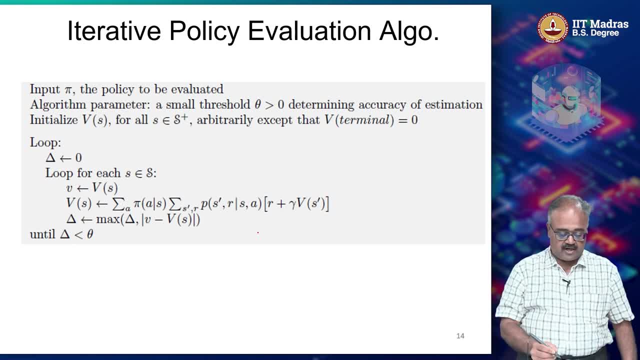 So just a few words. So let us look at it. So just write down an algorithm, So input is a policy, pi, and that is a policy that has to be evaluated, and then we have some threshold parameter, theta. I told you some 10 power minus 3 or something that we 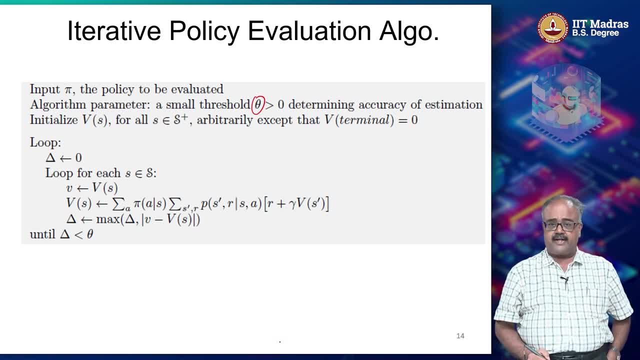 need to keep to stop it. So we have some small threshold, theta, that tells you when you have to stop, and then we initialize. well, you can, technically, you can initialize it to anything. initializing zero is just to tell you how the dynamic programming part works. 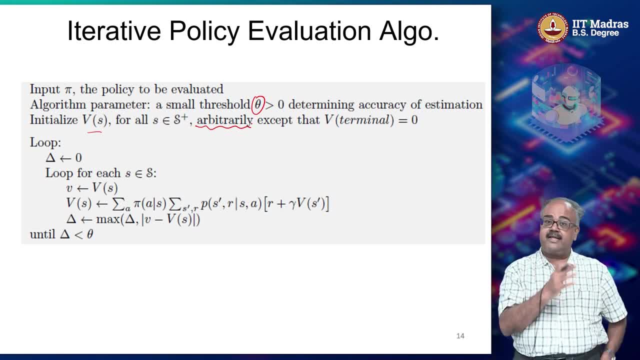 Algorithmically. you can actually initialize it to anything. it is still guaranteed to converge to the right answer. So you could do initialize it arbitrarily, or you could initialize E of s to zero for all s. But one thing I have to be very careful. 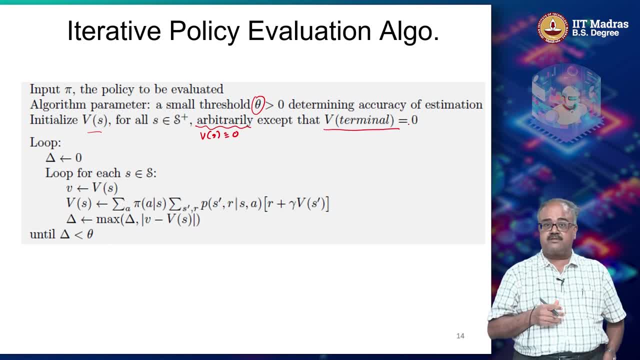 So the final state, if there is a final state in this whole process, if there is a final state for beyond which you cannot go anywhere, you have to hold it fixed at zero, Because it does not make sense to say that I have come to the end, there is no more action. 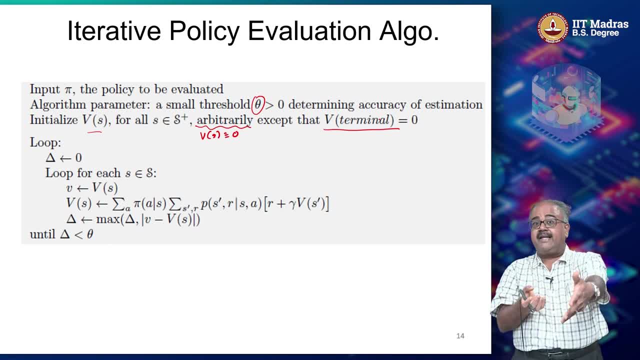 that I can take According to my policy, pi. but I am still getting rewards. I am still there is a expected future return. that does not make any sense, So you have to set your final value to zero. this is something that you have to remember. 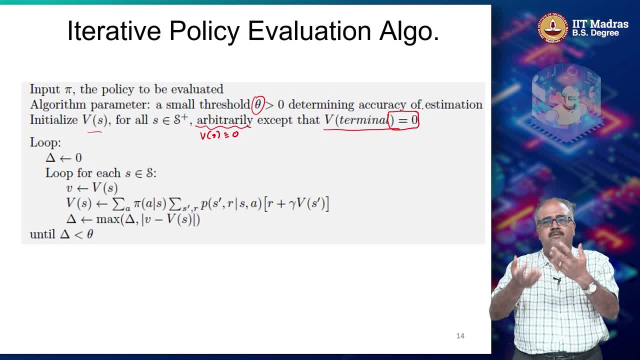 some later on. what happens is people kind of tend to forget this. as you learn more and more complicated stuff, you tend to forget the fact that the terminal reward or terminal value function has to be zero. So the last bit, you have to hold it to zero all the time. just be careful whenever your 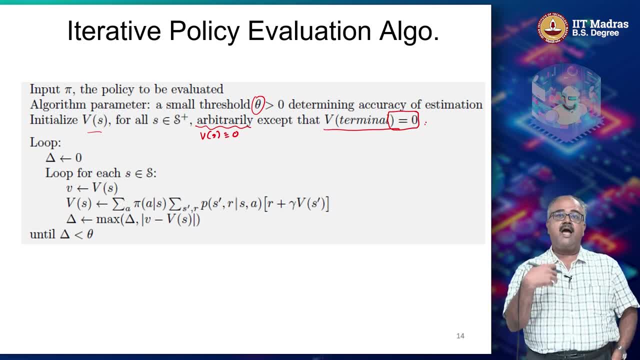 episode ends, The value function that you plug in has to be zero. you do not have to, you know, think of a specific terminal state and use a value zero for it. It could very well be that whenever your episode ends, instead of doing this, you just use r. 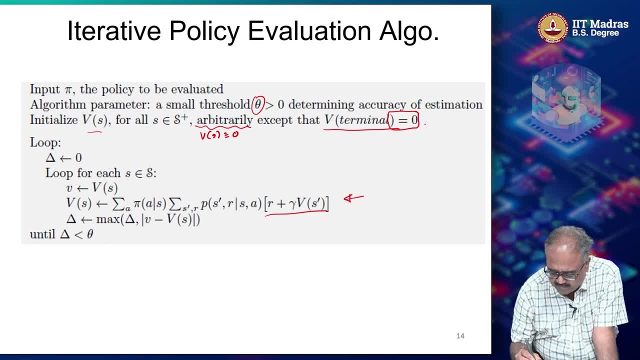 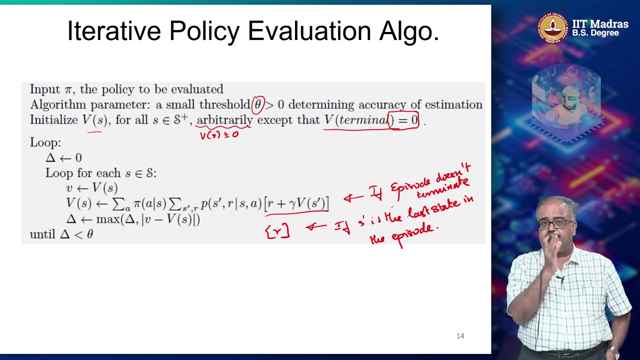 So you do this. if does not terminate, Okay, Okay, Okay, Okay, Okay, Okay, And you do this: the reward for the next date or if s prime is the last date in the episode. So you do not. you are updating s. 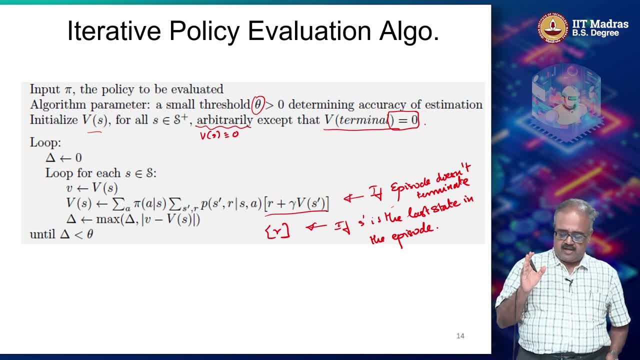 So s prime is the last date in the episode. Then you do not use v of s prime in your update. it should just be r, right. In fact I recently, when I was teaching my RL class in person, right? So I actually discovered that a lot of students were actually using a library. that is out. 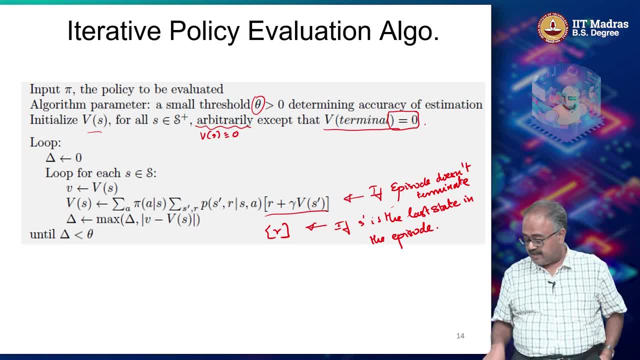 there that does not do this and it turned out because of this. they were getting wrong answers and they are doing this simulation, So you have to be careful about it right, even though the algorithm describes it like this. So remember that if you come to the terminal state in the episode, and if it is truly the 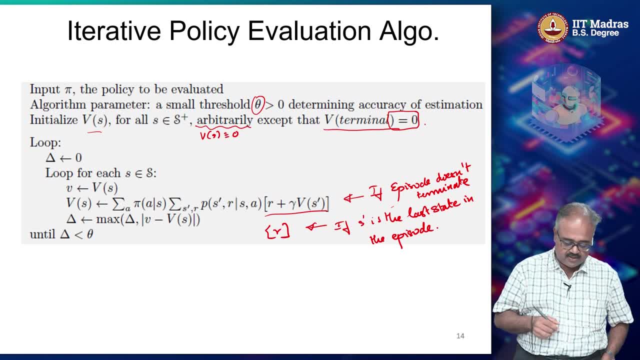 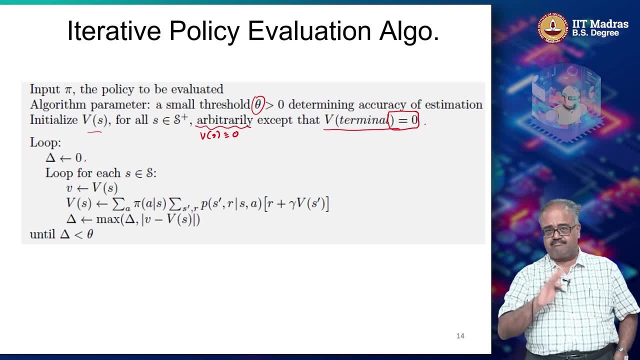 terminal state, not because you stopped training, then you should use this as your just remember this as an aside. So now, what we do? we start off by, you know, setting some parameter: delta. I will tell you what delta is in a minute. we will set delta to 0 and then for each state s, then we basically 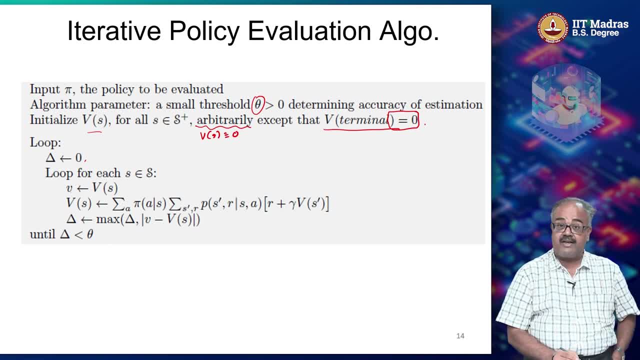 start doing this. So we take the old value of v of s, that is the last value in the previous iteration. So this is basically the kth value. So you take vk and store it temporarily in this variable v and then you use your update. 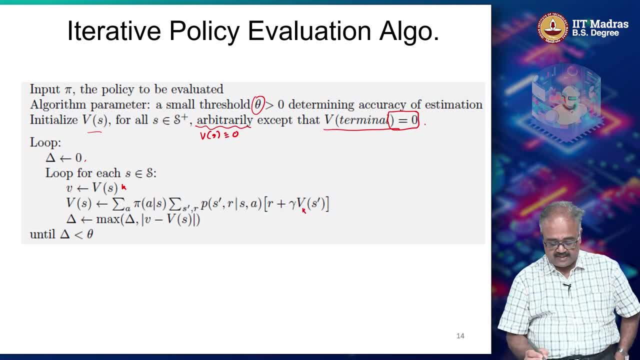 rule. So this is essentially the update rule that we saw earlier. So this is basically k and this is k plus 1. that is what we did. this is k and k plus 1.. So after you have done that, you compute the difference between the old v, vk and this. 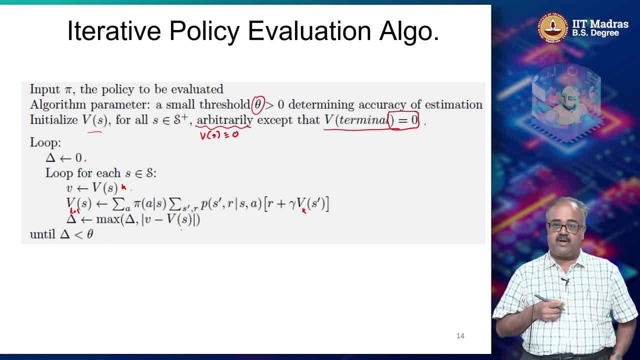 is the vk plus 1.. So you compute the difference between vk and vk. So you compute the difference between vk and vk. So you compute the difference between vk and vk plus 1 right and see if it is larger than the largest difference you have seen so far. 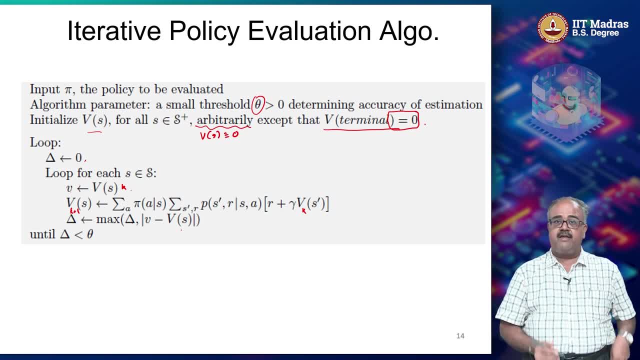 If this is larger, then replace cap delta with this. if it is not larger, then leave delta as it is right. So basically, use the max right, then keep going until your capital delta becomes smaller than your threshold that you had earlier theta right. the theta could, like I said, could be. 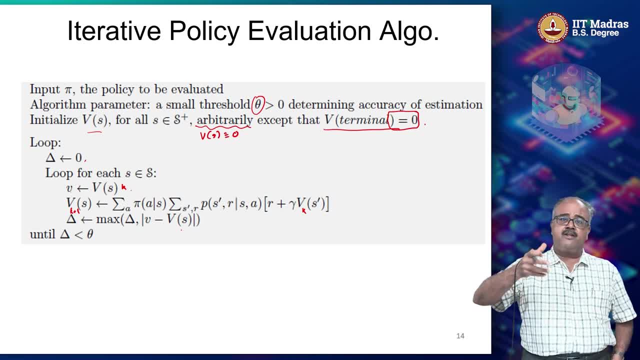 10 power minus 3.. So keep iterating until the maximum difference you see from k to k plus 1.. So k plus 1 is less than 10 power minus 3.. So that is basically when you stop. right, this is, this is the stopping condition. you keep. 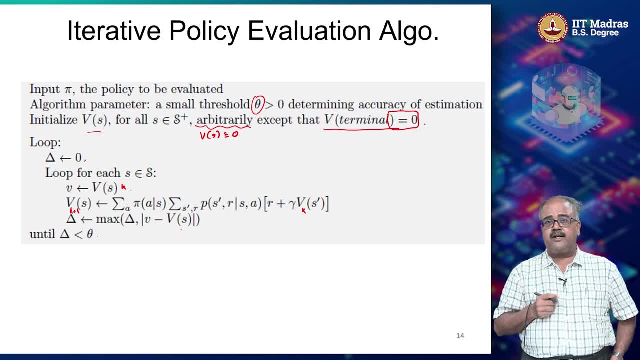 iterating. otherwise. right and again- I am not going to get into the proofs today, but you can watch it on the videos- that this is guaranteed to converge to a solution. right, it is guaranteed to converge and stop at some point, because this equation that we have here is what is. 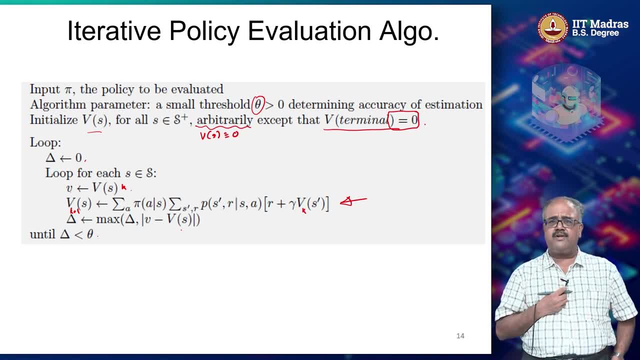 called as a contraction operator, right? I am not going to get into the details of it. you can look it up if you are interested, right? So you can think of it as so the reason we are doing this funky thing, right? So, why we are putting a v here and then comparing the capital V with the small v and all that. 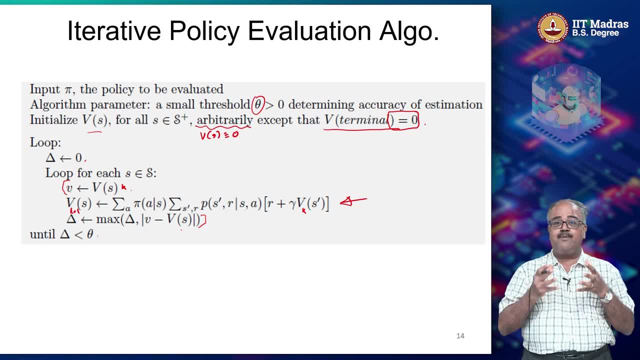 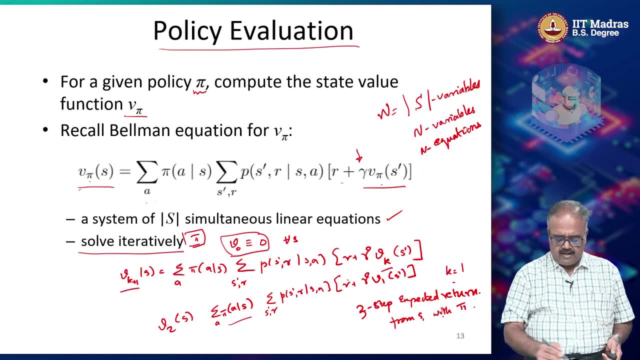 is because we are trying to do this in a slightly more efficient manner. right, If I had done this? right, if I had done it like what I talked about here? right, have a v k here and a v k plus 1 here, and so on, so forth. 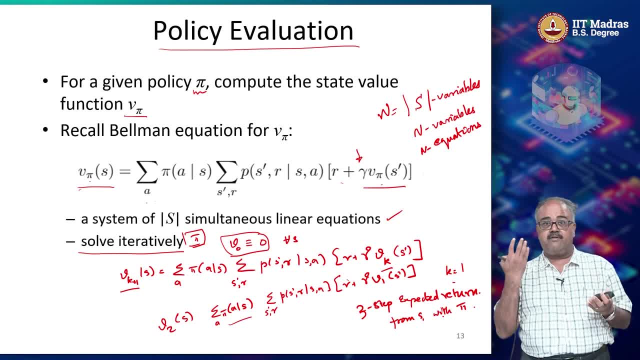 You would need two copies of v, right? we need the k copy and the k plus 1 copy. So for us to do that will be wasteful of memory, right? So doing this update, right? so this is called a synchronous, this is called synchronous. 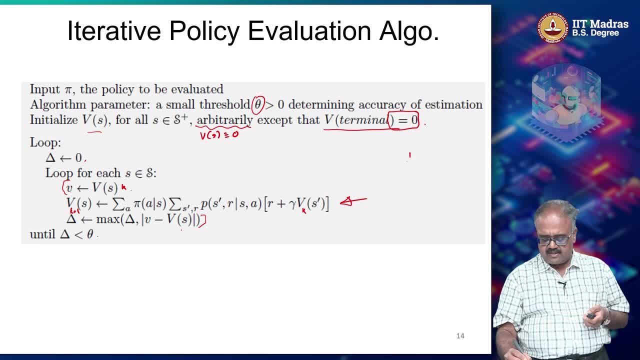 update, right. So this is some. this is, you know, this is in place updates. in place update means I am not making two copies of v k, v k plus 1.. I am just changing the one copy itself, right? I am just changing one copy of v k to v k plus. 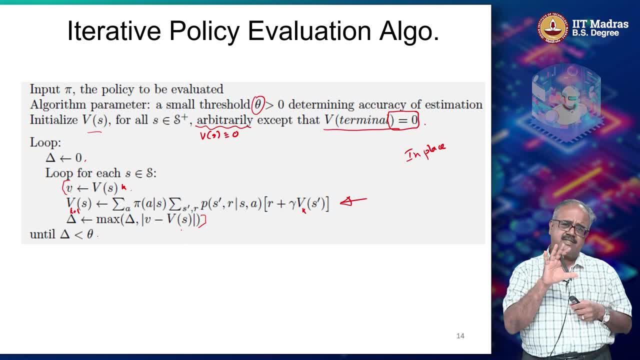 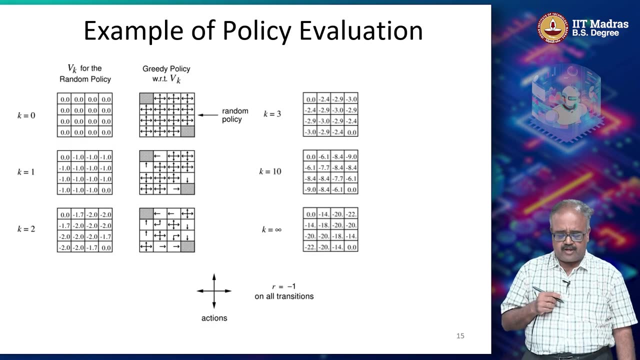 1. So this algorithm is a little efficient algorithm, but it also hides the small fact. think about it. So I will. I will show an example. I will show a numeric example and then come back and talk about this algorithm, right? So the numeric example is going back to the greedy policy that we had earlier. sorry going. 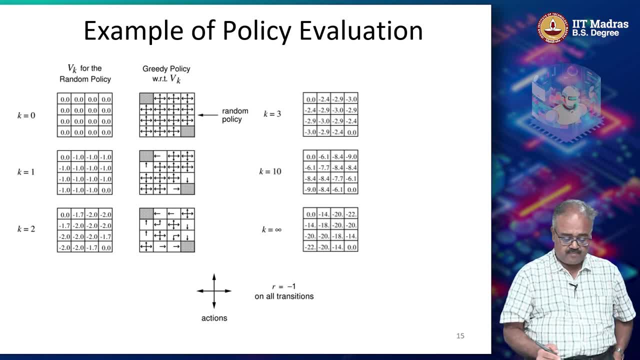 back to the random policy, Sorry. So here is a grid world right and it has two absorbing states. these two corners are absorbing states for the grid world, So go into either one of them and then you stop right, and then we are talking and you. 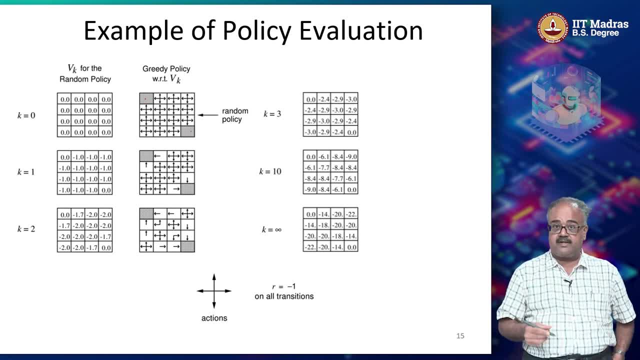 get a minus 1 reward for all transitions until you stop. So the optimal way of solving this problem is to get to one of those corners as quickly as possible and not move from that right. but then we are going to talk about a specific 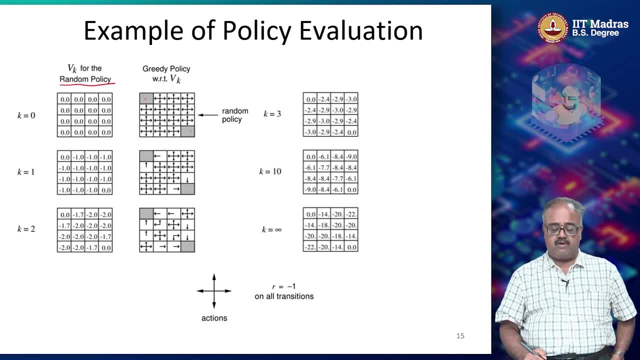 policy pi right. So the specific policy pi here is a random policy. So what we mean by the random policy? that you could go in any direction with equal probability. So this is basically what the random policy is right. So there is a 1- 1- 4 probability of going up: 1, 4 probability of going down: 1, 4 probability. 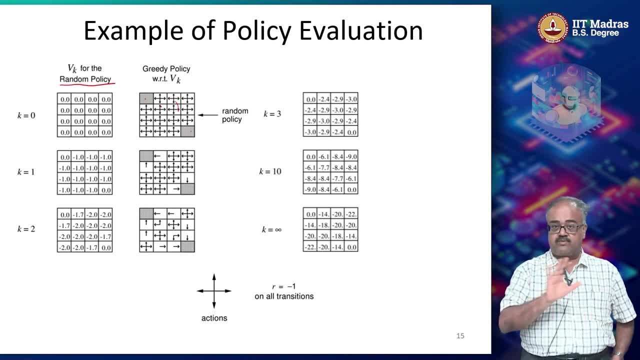 of going left: 1, 4 probability of going right in all the states. right, that is what a random policy is, right. So I start off with v k being all 0s, like I was telling you earlier. So we start off with v k being all 0s. and what is v k 1? v k 1 is expected. reward you. 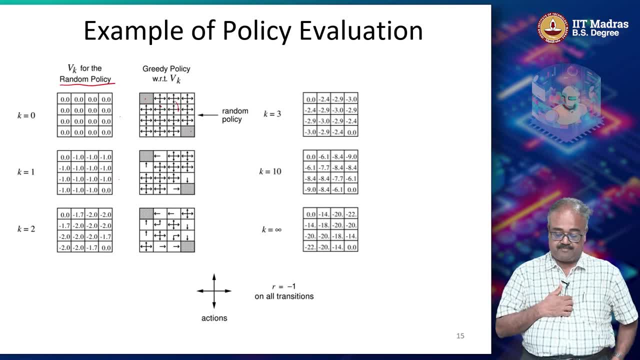 are going to take. So v k 1 is expected reward you are going to get for taking one step right. so what happens when you are taking one step? it does not matter, because one step you are going to stop right. So for that one step you are going to get a reward of minus 1, so you are not going 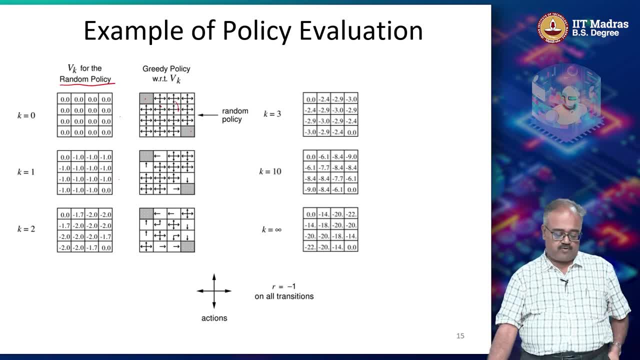 anywhere. So you just take one step and you stop and you are getting a reward of minus 1, right? So does not matter which step you took, whether you went left up, down or right- you are always going to get a reward of minus 1.. 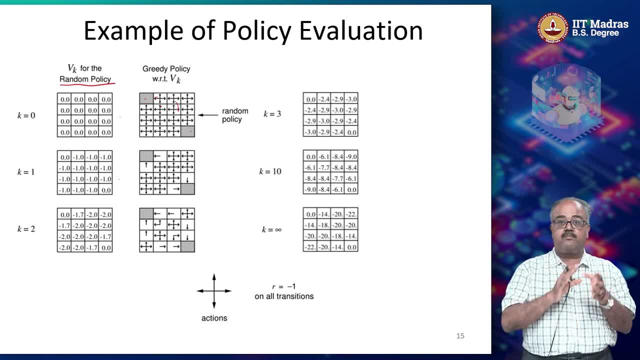 So you are going to get minus 1 into 1 half, Minus 1 into 1 fourth, minus 1 into 1 fourth and so forth, and so the total is going to be a minus 1.. So you can see that for that one step function all the states. you get a reward of minus 1. 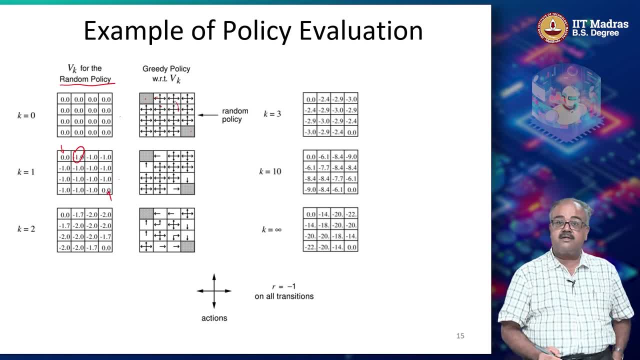 right and remember: these two will stay 0 because they are terminal states. you do not move from that, So their reward will stay 0.. So I hope it is clear why all of this is minus 1, taking one step. it is not that because 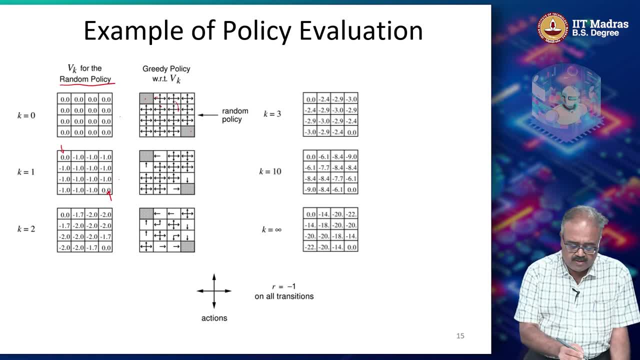 you are getting a reward of minus. it is actually a little bit more complex. answer, right. So because? why? let us let me write out what happens here, right? this is the easy case, so I can easily write out. So remember, I am going to sum over all a pi of a given s right. it does not matter what. 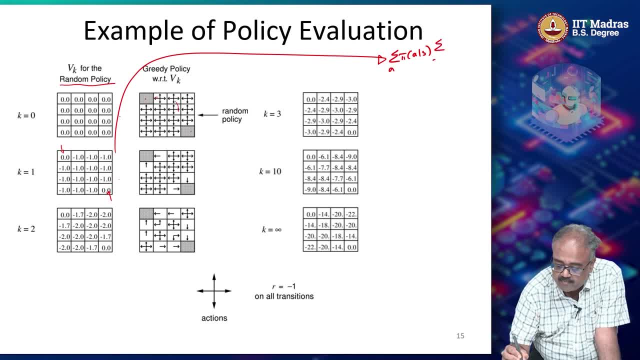 s is. this is going to be always 1, fourth right, and then I am going to sum over all s prime and r probability of s prime r given, and then r plus comma, v of s prime. So v of s prime is gone, so it is 0. so I do not have to worry about it. let us worry about 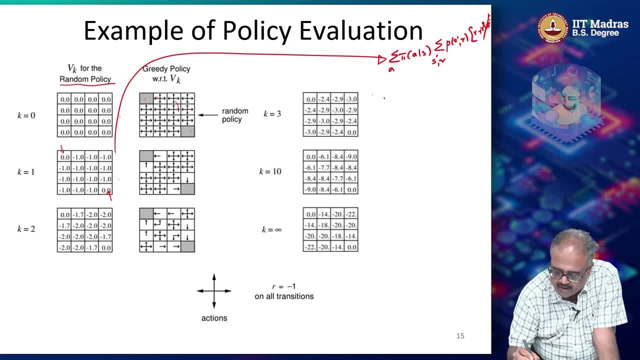 the other one right. So action say north, right, so I am going to take north, so, which is like 0.25 probability, right, and what is the probability I am going to end up anywhere. so just one step right. So basically I am here, I go north, I end up in the same state, right, I end up in the same. 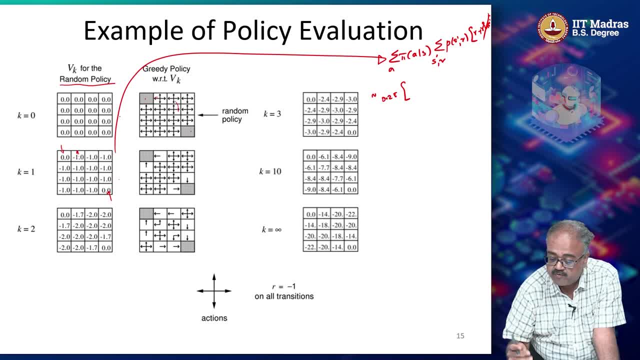 state: with probability 1: right, there is no question about it. and I get a reward of minus 1 with probability 1: right. and what about gamma v of s prime? So what about gamma v of s prime? We do not care about it. so this is basically summation over s prime, which is probability. 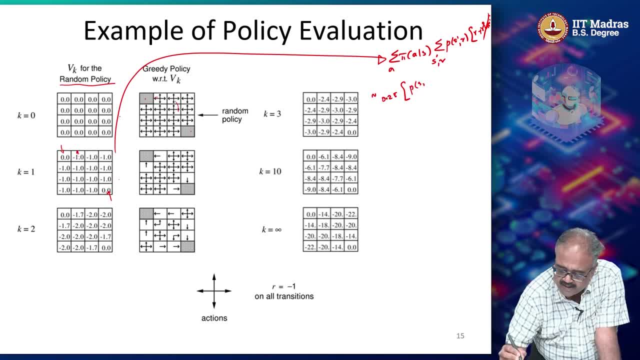 of the same state right probability of s comma r, which is minus 1, so minus 1, and that this combination has a probability of 1. everything else has a probability of 0. So it is 0.25 into 1 times minus 1, plus 0.25. 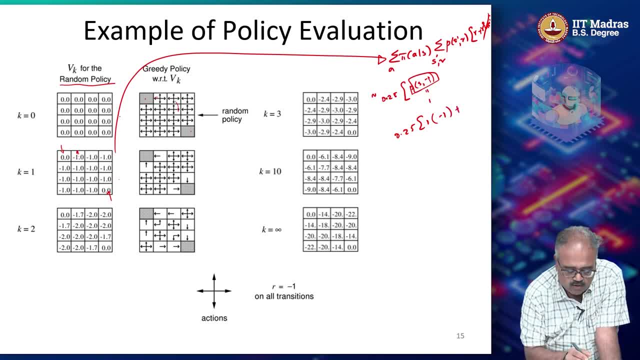 Okay. So what about gamma v of s prime? We do not care about it. Let us say: go east. right, yeah, go east. so go east from here. so again, that is a 0.25 right times. the probability of going east will put me in this state. so that is s prime, that is. 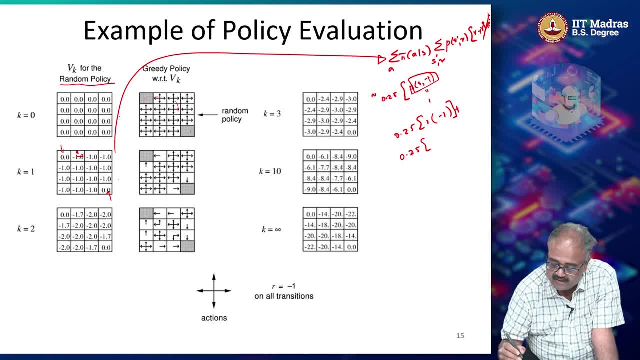 only one, that is, only state that has a probability of occurring, and then the reward is minus 1.. So I will have probability of 1, of minus 1, plus gamma times the value of this state, which we already know is 0, right? 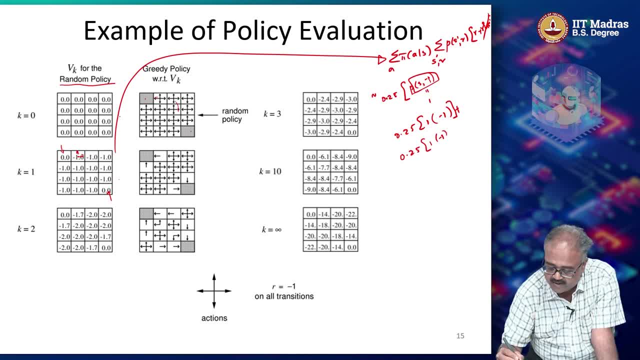 Right, So we do not have to worry about it. so again, it is minus 1, right, it is like that this is basically what will happen. okay, so, even though it just looks that, but this is how the computation happens, right, it is just one step. reward, it is a minus 1, but there are 4 possible outcomes. 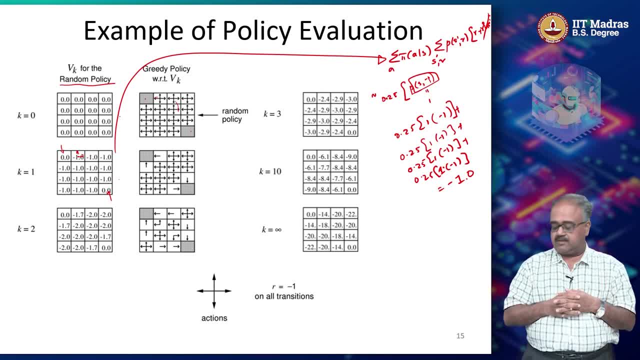 because there are 4 different actions. I have to consider all the possible outcomes and then basically end up getting a minus 1.5.. Okay, So this is a minus 1. right now, when you go to k equal to 2, what happens right when k? 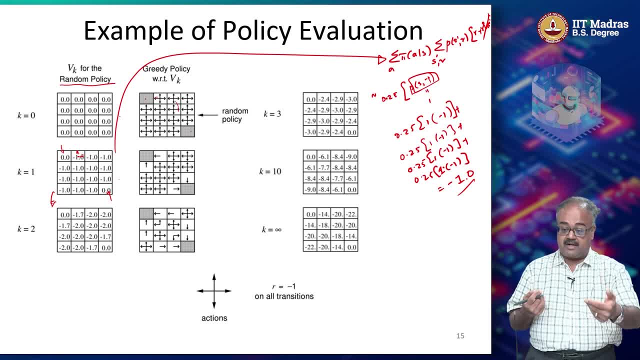 equal to 2, again you have to do the same thing. but now you cannot ignore your v of s prime. you have to use the v of s prime also, right? So what happens here? when I try to move up, right, I will stay in the same state. so my 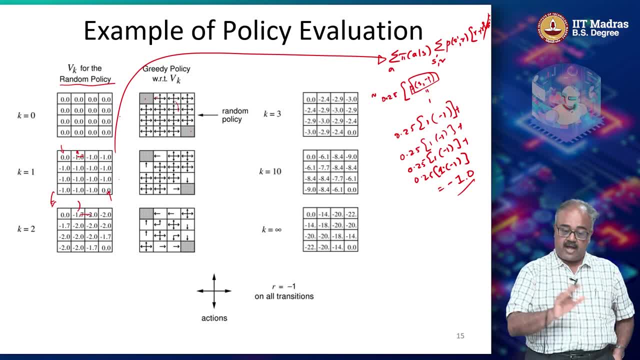 v of s prime will be minus 1. likewise, when I try to move here, I will move, but that that state also has a minus 1.. So that will be again minus 1.5.. Okay, When I try to move down, I will move. it is a minus 1. then I try to move west. what happens? 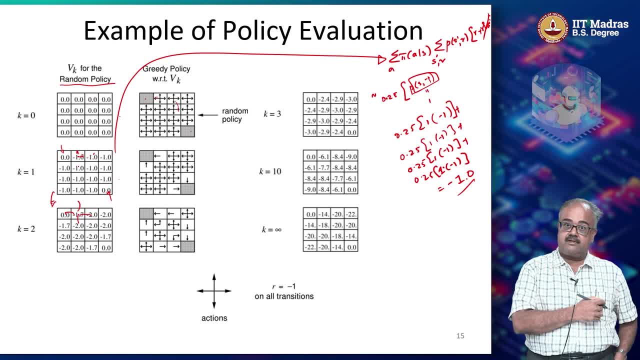 I actually go to the terminal state right, and that will going to have a reward of 0. So I am going to get a minus 1 plus a minus 1 minus 1 plus a minus 1 minus 1 plus a minus 1 and a 0. actually, it is not a 0, it is a minus 1 plus a 0, so that is a minus 1 as well, okay. 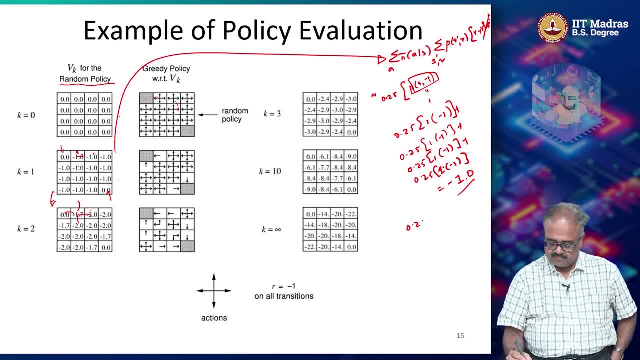 So I am going to get 0.25 into minus 2.5.. Okay, So that is a minus 1.5.. Okay, So I am going to get 0.25 into minus 1, plus 0.75 into minus 2.. 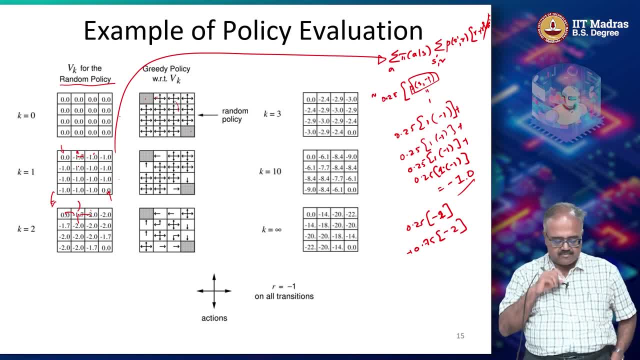 Okay, So rounding it off, you get basically, you get 1.75. that is basically what has happened. So k equal to 2. it is like I take one step and then I take another step. where do I end up at? So that is basically what we are asking, right? 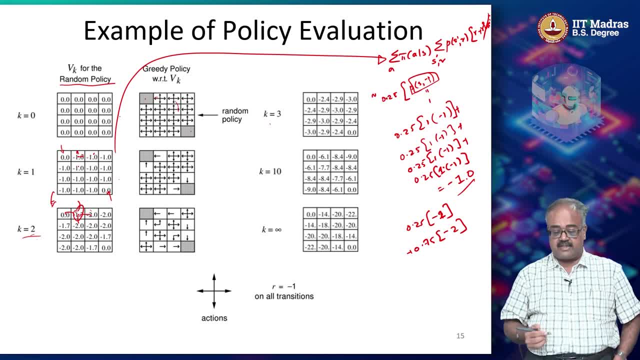 So that is k equal to 2. likewise, k equal to 3 is what happens with the 3 step policy, and so on, so forth, Until you hit k equal to infinity, which is where- which is a final value function. So this is basically the p? pi corresponding to the random policy. 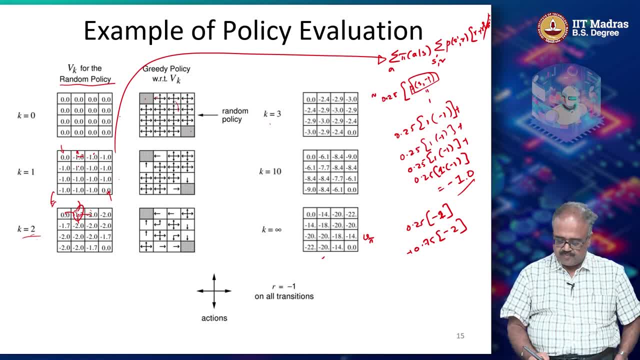 Okay, Does that make sense? right, and we can work on more complex problems. and you know, in one of the later videos you will see a slightly more complex illustration of value iteration, policy, iteration and different ways of solving this problem. Okay, So this particular computation that I demonstrated to you is essentially implementing these set. 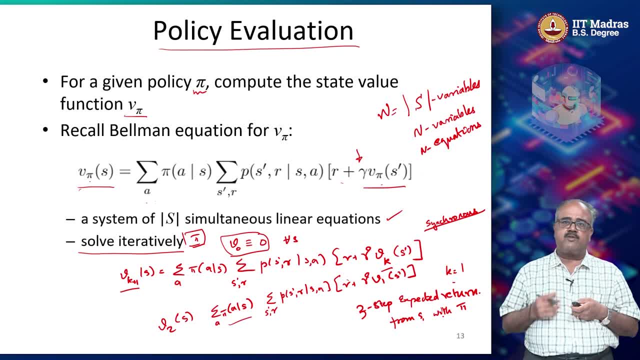 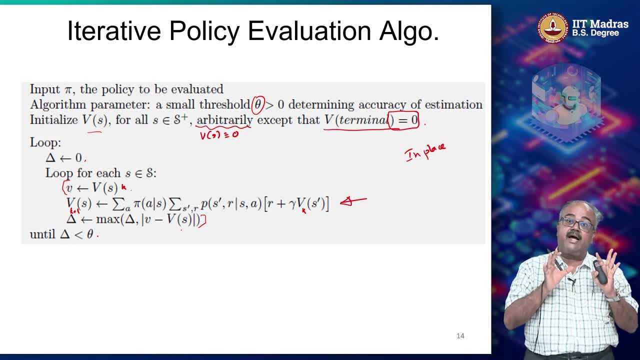 of equations here, Right So where you have k on the right hand side and k plus 1 on the left hand side. Right, This algorithm, Right, This algorithm that you see on the screen is not quite that. it is slightly more complicated. 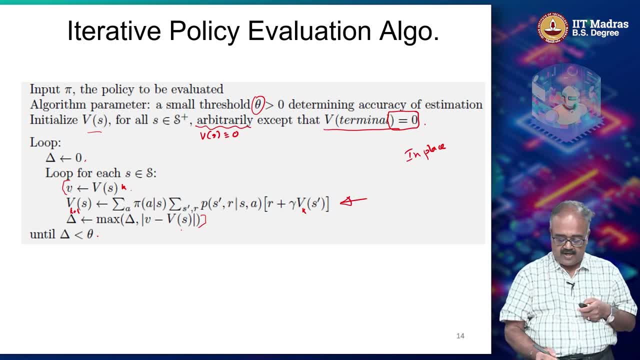 because when I am looking at the first state, Right, I will be using k, But what do I do? I update the v of s to v k plus 1 of s, Right. That is what I do here. So when I come and look at, when I come and look at the second state, when I come and 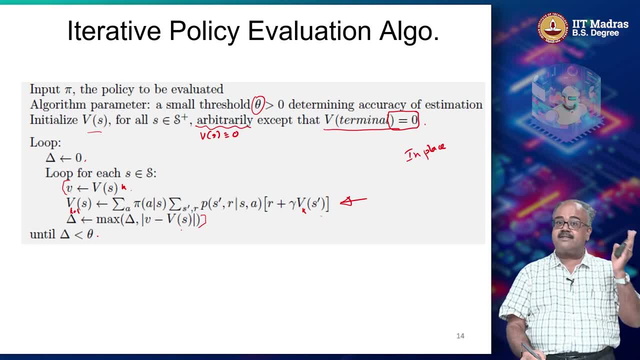 look at the second state. but if I have to access s 1 on the right hand side, I will actually be using v k plus 1 of s 1, because I have already updated the value when I looked at s. See, I start from s 1, then I go to s 2, then I go to s 3, then I go to s 4.. 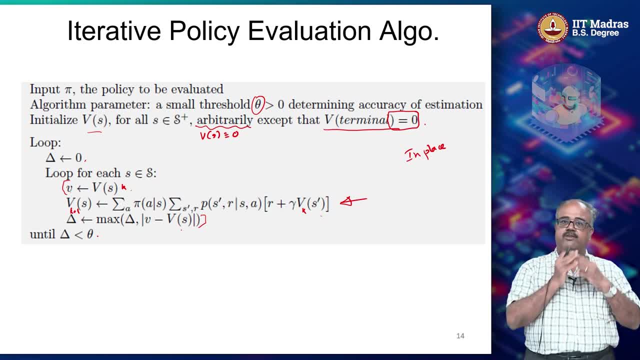 Right, So s 3 is how I am looping. So when I first come to s 1, I am going to compute v k plus 1 of s 1.. Right, When I go to s 2, if I have to access v of s 1, what I will have there is actually v k plus. 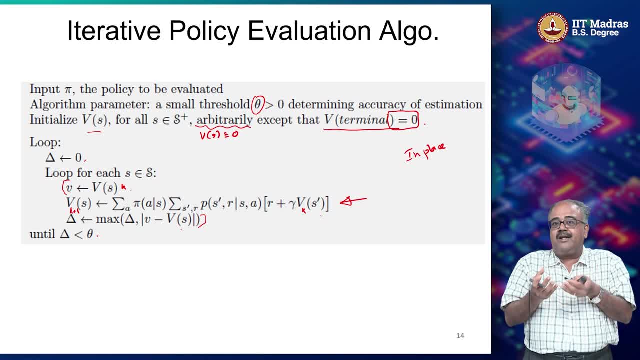 1 of s 1. Right, So it is not like I take k to the right hand side and get k plus 1 on the left hand side. Depends on the order in which I am doing the computation, Right When I am actually looking at the last state, like, say s n. 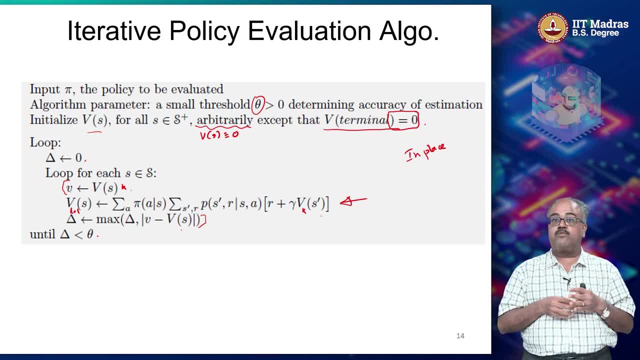 Right, So the other state, except s n, will have v k plus 1. s n alone will still be using v k, Right? So it is a slightly kind of a asynchronous computation. is what is implemented in this algorithm, Right? So it may make sense. 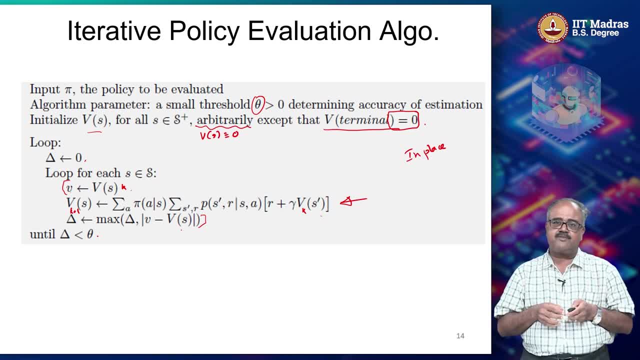 Right. So this algorithm is a little efficient way of implementing it, but it does it in an asynchronous manner, does not quite match the k, k plus 1 explanation that we have been giving Right. So we have ensured that this implementation also will converge to v pi eventually. 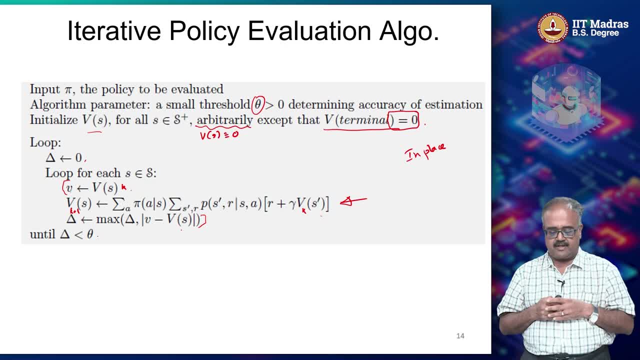 Okay, So that is. that is basically it. just that makes it a little bit more efficient. Thank you very much.